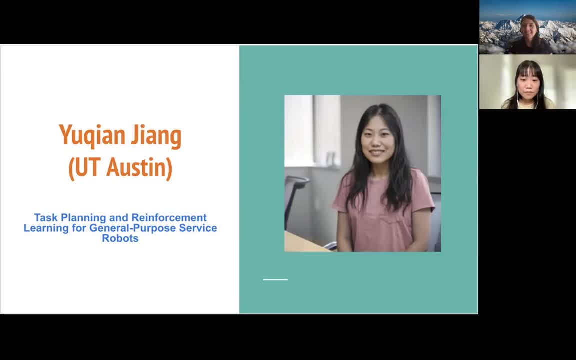 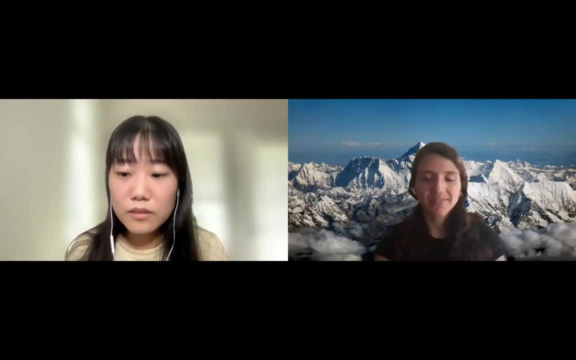 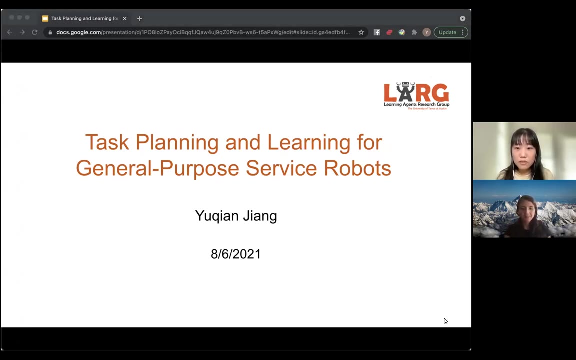 am gonna pass it on to you, kia. thanks for the introduction. i'm gonna share my screen. yeah, okay, hopefully it's working. yeah, yeah, cool. well, thank you for inviting me to give this talk. i'm yu qianjian and i'm very excited to present our work towards task planning. 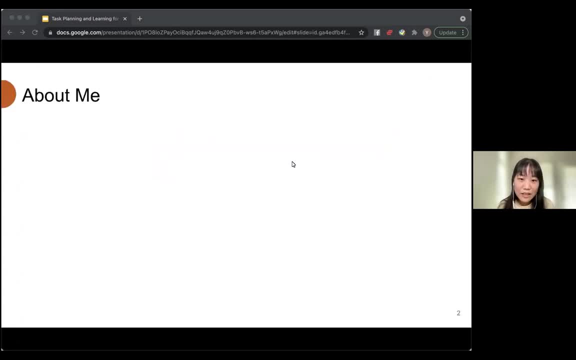 and learning for general purpose service robots. um, just a little bit more about myself and the robots that i work with. i'm a phd student currently finishing my fourth year of my master's degree and about to start my fifth year. like nations, and i'm advised by professor peter. 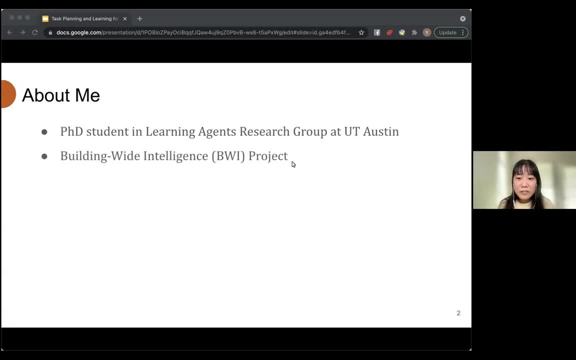 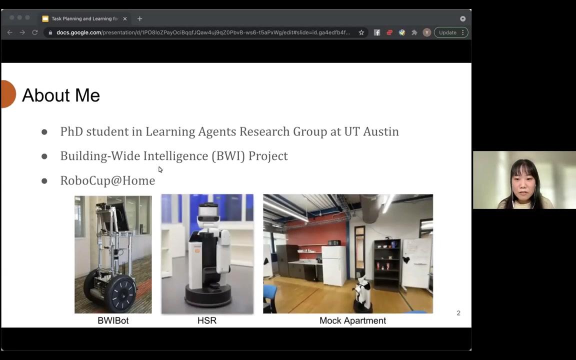 stone um. i have been working on the building white intelligence project, where we have a fleet of these mobile robots in our computer science building, and also the current leader of our cup at home team. we just finished in the third place in the virtual competition this year and but usually the competition uses these physical um hsr robots and they 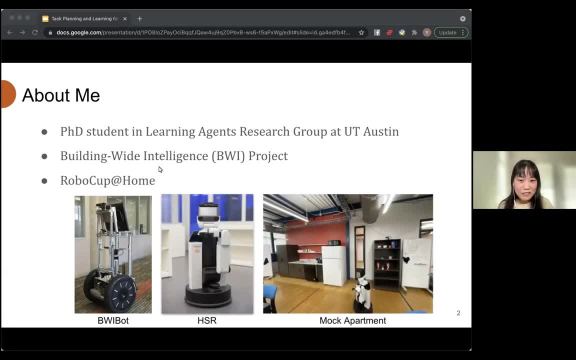 have a lot of experience, and we also got this new lab space that looks like a home environment. you know we're new robotics building, so that's very exciting and um. so these are the service robot platforms that you will see in this talk, even though they have slightly 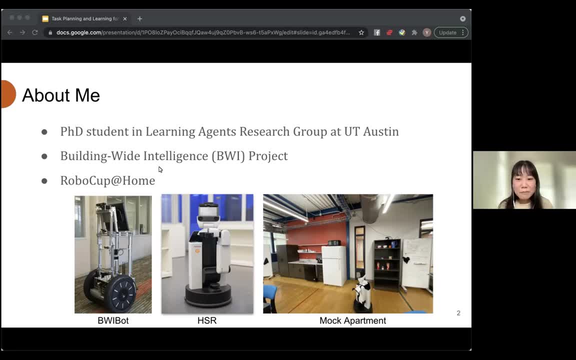 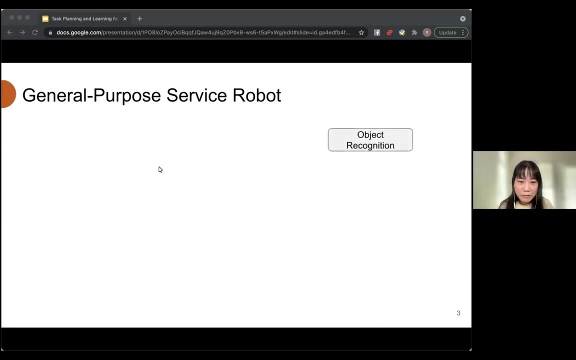 different target environments and different capabilities. we have been building one planning framework for both of these robots and environments and today i will talk about our work towards this framework. so to build a service robot, of course you will need a bunch of capabilities like object recognition, manipulation, navigation, natural language. 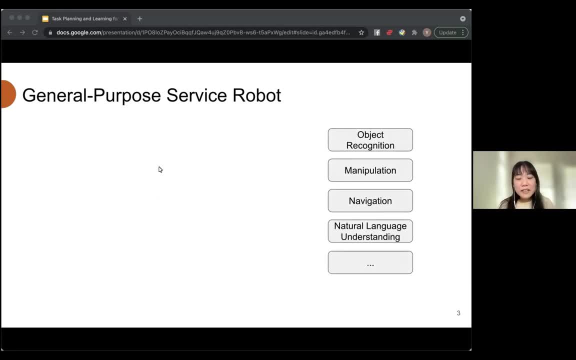 understanding and so on. um, and we've seen a lot of recent progress in all those areas, especially with, you know, deep learning based approaches. before a general purpose service robot, it's also essential to be able to reason about the task and sequence these skills when given user requests like bring me coffee, and i'm generally interested in closing this gap. 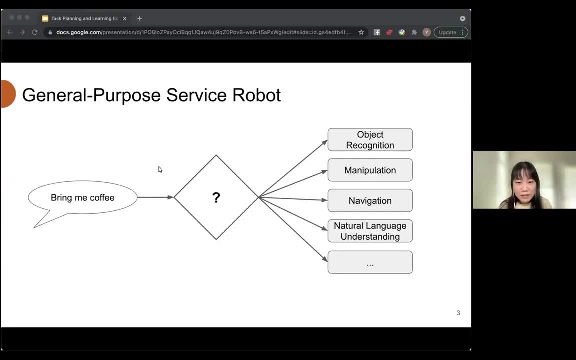 between the robotic skills that we're testing in lab conditions and skillable, robust, general purpose service robots that can work in realistic environments. um, in general, there are, you know, two classes of approaches to this problem. there's symbolic planning, or automated planning, that generates the sequence of actions based on a model or a description of the task, and 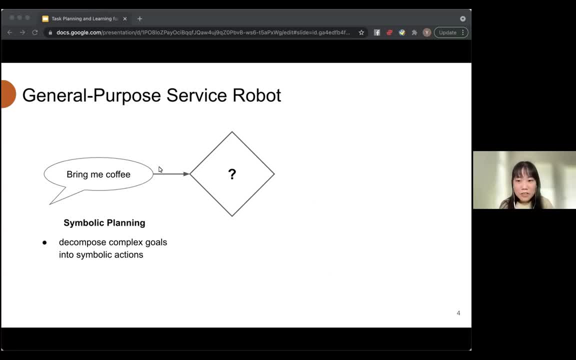 actions. the advantage is that we get a natural decomposition of a complex goal, um, into symbolic actions. of course, the disadvantage is a need to be able to work in the same environment, and there are a few issues that we can address um, but i want to start by emphasizing that the problem is that if we don't have the right 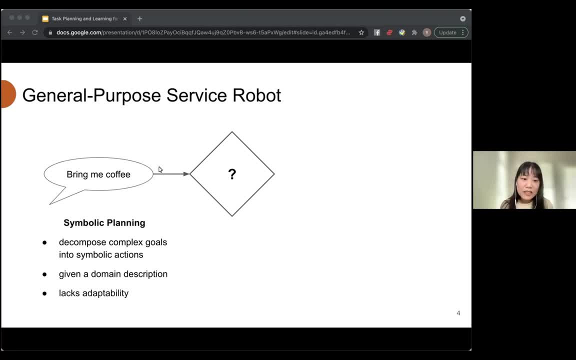 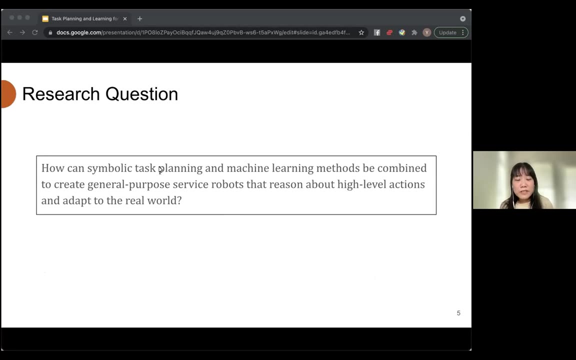 needs a domain description and it lacks adaptability if the model is wrong. There's also machine learning, which can be model-free and can work on a raw sensory input, but it requires lots of data or experience. So the high-level research goal is: 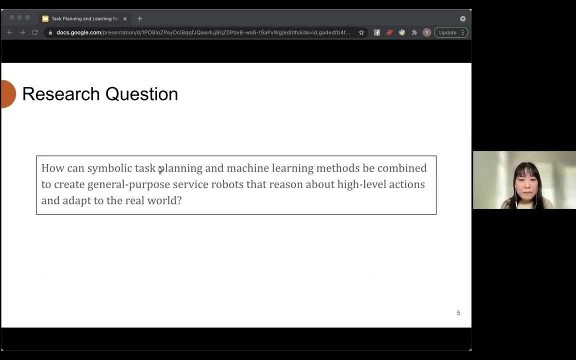 that we would like to combine the strengths of symbolic task planning and machine learning methods in this framework to reason about high-level actions and adapt to the real world. And in general, we approach this question from two directions. First, we will address challenging scenarios. 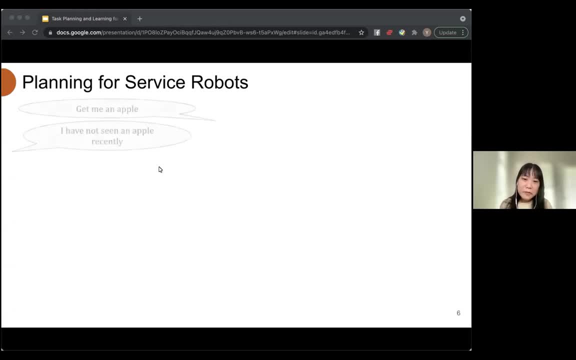 for robot task planning or task motion planning. Scenario one: suppose the user asks the robot to get an apple, but the robot does not know where the apple is. We have introduced an approach to plan with no-sounding objects. Scenario two: on the way to deliver your apple. 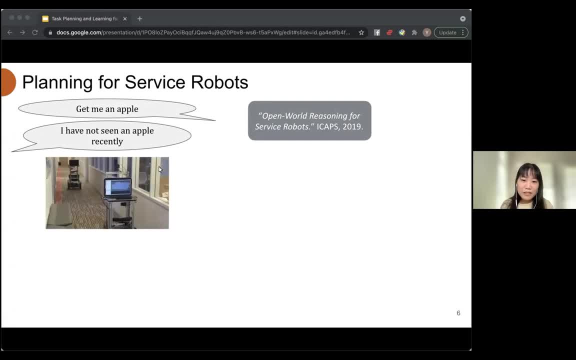 the robot runs into another robot in the corridor. When there are other robots in the environment, they can have conflicts like this, blocking each other in a corridor, and they can form synergies, Like one of the robots could go ask for help to open the door or something. 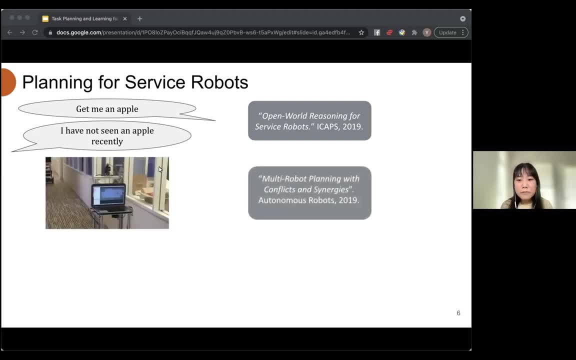 And we've developed a framework for the problem of multi-robot planning with conflicts and synergies. Scenario three: there could be many valid paths for the robot to bring the apple to you and the dynamic environment changes. the environment changes to bring the apple to you and the dynamic environment changes. 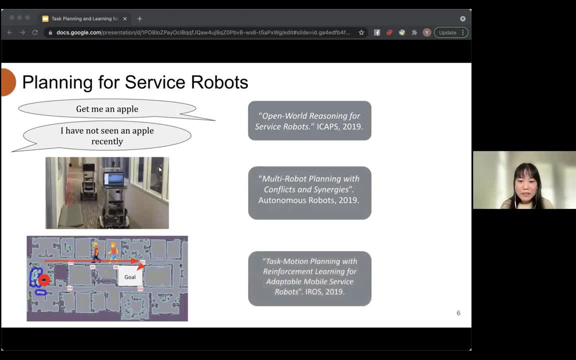 to bring the apple to you. and the dynamic environment changes the cost of those plans. So we've proposed a task motion planning framework which iteratively plans and learns the costs of navigation actions. And even though these scenarios or challenges may seem a little disjoint- or maybe they 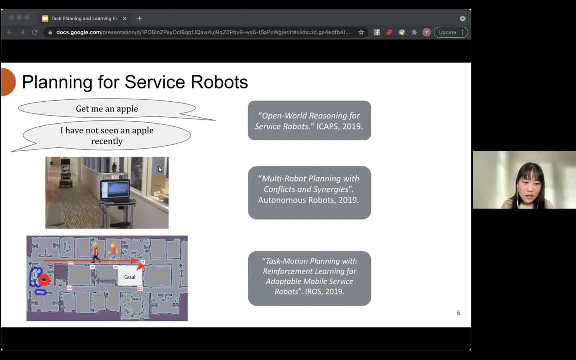 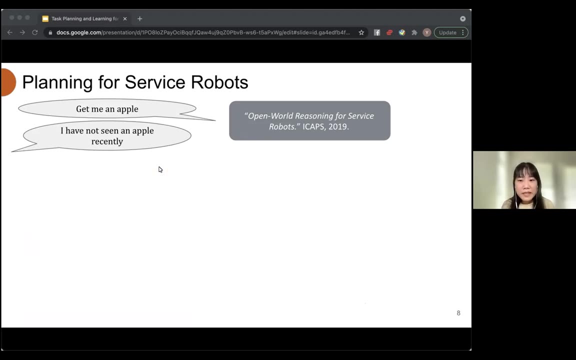 can be individually addressed by other techniques. our goal again is to build a unified planning and execution system so that a general-purpose service robot can handle all those scenarios. First I will present our work on planning in the open world with unseen objects. 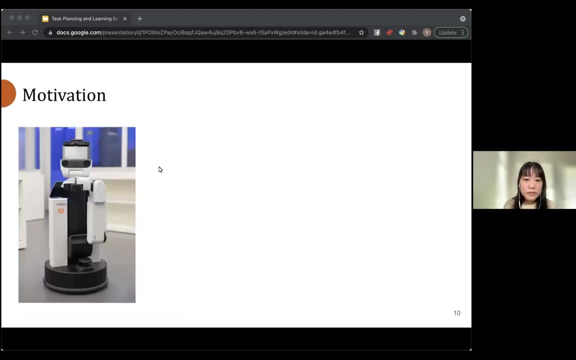 This was joint work with Nick Walker, Justin Hart and Peter Stu. When you get user requests like get me an apple from the kitchen, if you know where the apple is, it's easy. You can just use existing symbolic planning approaches. 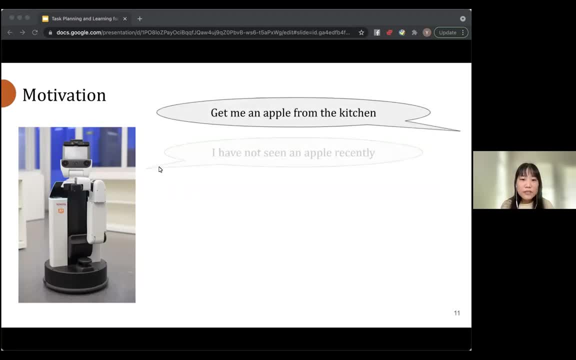 to generate a plan like this. However, if you don't know where the apple is, it's difficult for existing task planning approaches, because most of them adopt this close-world assumption, which means that everything the robot needs to accomplish is already represented in its knowledge base. 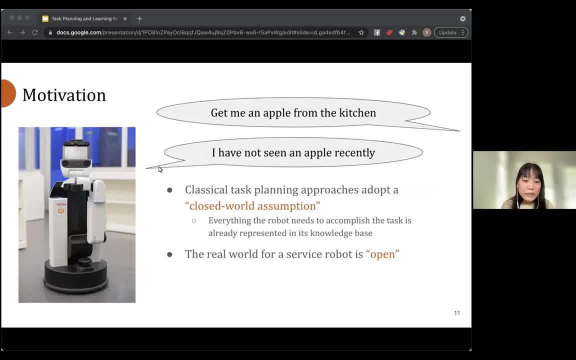 But the real world in general will violate that assumption At any time. the next command the robot receives might refer to an object that is not currently in its knowledge base or the initial space. So it's a little bit more complicated than that. So it's a little bit more complicated than that. 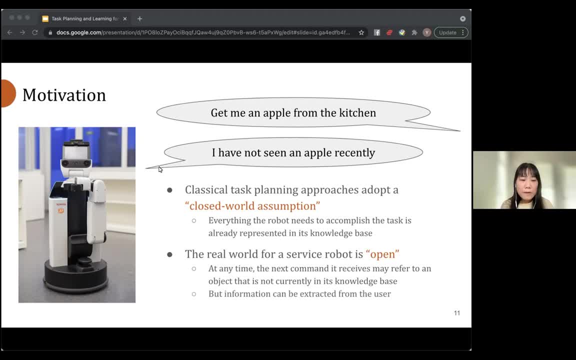 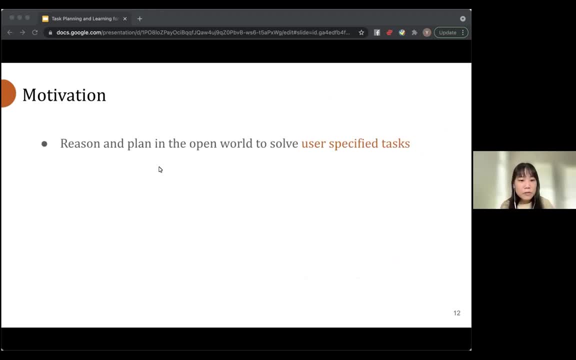 So our motivation is to reason and plan the open world to solve user-specified tasks, And we want to leverage the user's implied hypotheses of unseen objects so that we can just use generic closed-world planners, And we also like to use the same method. 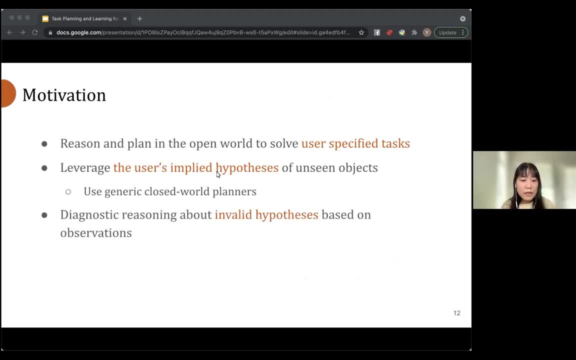 to do diagnostic reasoning about invalid hypotheses when the robot has made observations in the real world. And, of course, knowledge reasoning and planning techniques have been widely applied to service robots. Our work is directly motivated by the test in RobotCup at Home. 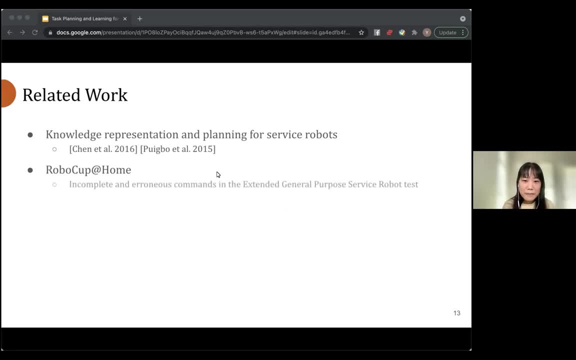 where the robot can be given complete and erroneous commands. Also, open-world planning is not a new area or concept. There are many kinds of openness of the robot's knowledge or the planning domain and some of them have been studied In this work. we target this common scenario. 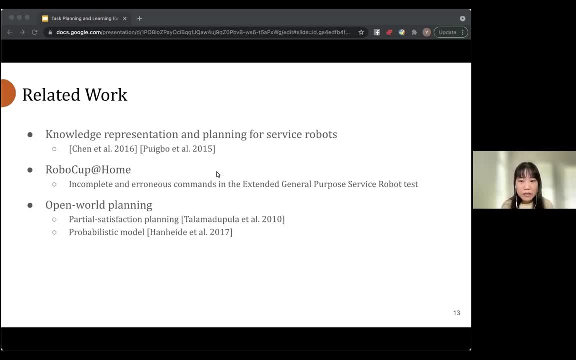 where the robot hasn't seen something that the user knows about and can therefore form hypotheses about those objects based on what the user is saying. So here is an overview of the steps in our approach. First, we close the world by representing unseen objects referred to by the user. 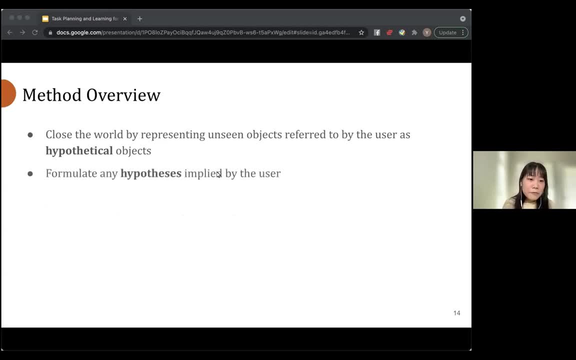 Then we formulate any hypotheses implied by the user And we model special realizer actions to allow feasible plans to be generated with hypothetical objects And we propose the diagnostic reasoning approach to identify hypotheses that are inconsistent with observations made during plan execution, so the robot can have useful information. 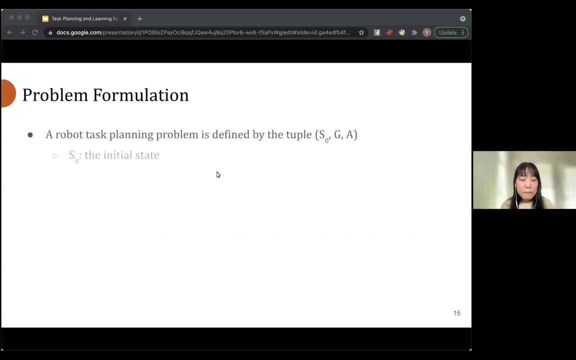 to report back to the user Before we move on. problem formulation looks very familiar for anyone familiar with task planning. The only difference is: in this case we have an open world where the information necessary for the goal can be missing in the initial state. 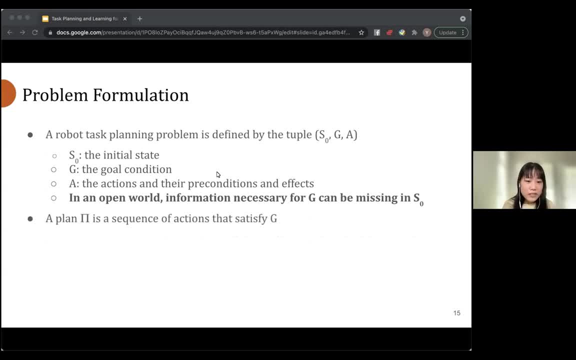 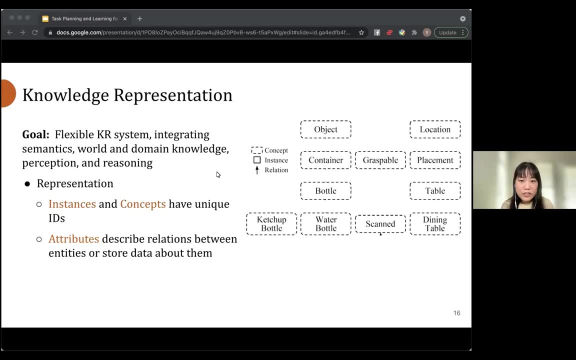 And we're trying to generate a plan that's a sequence of actions that satisfy the goal condition. Here is a visualization of our knowledge representation system. that's sort of a core. The data is not a single component in the whole solution. The representation has instances and concepts that have unique ideas in a database. 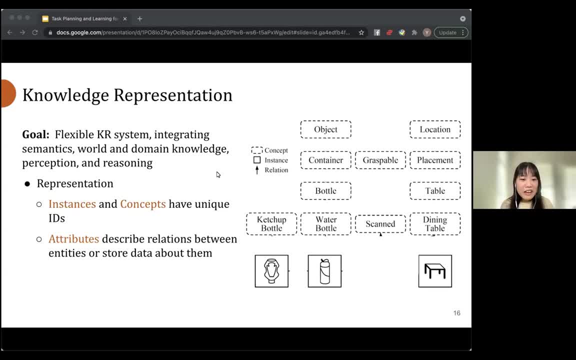 So an instance is like when the robot saw a concrete instance of a ketchup bottle, and there's also the concept of the ketchup bottle or the concept of a table represented, and those things are linked together by attributes that describe relations between entities or 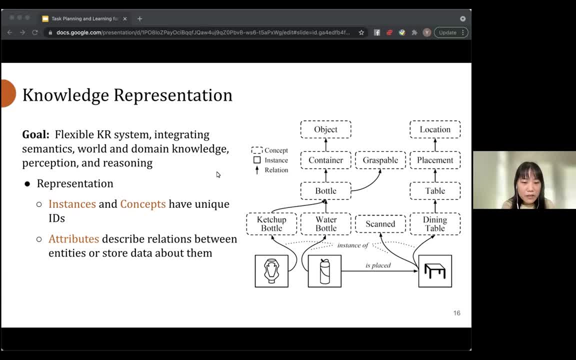 the data about them, Like, for example, this water bottle is placed on the dining table. A quick question So: do you build this knowledge representation or is it given to you? You have these attributes basically beforehand, or does the agent, as it goes and explores, it builds this graph? 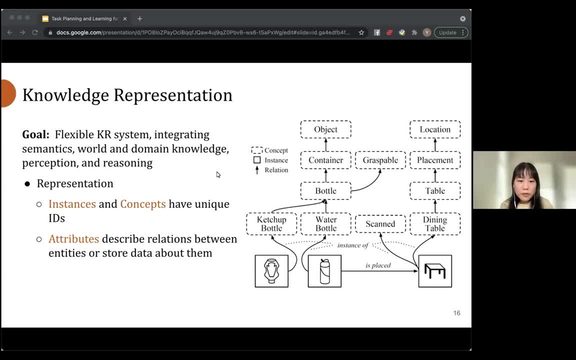 This is partially built by the agent using its. We assume there's already a perceptual module that can do object detection, like YOLO, and part of those concepts are sort of given. So this is a hybrid of what's already given and what the robots detect in the environment. 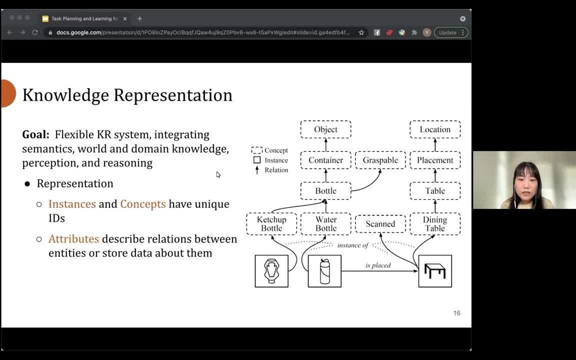 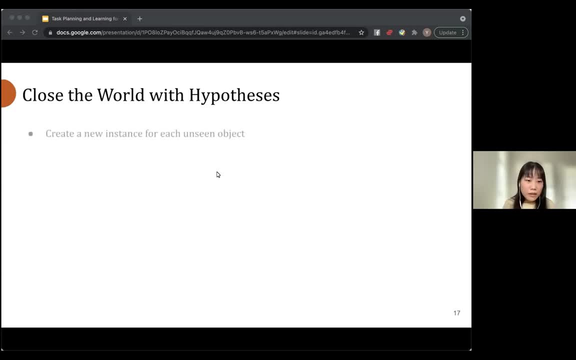 Like those instances are all detected. I see, Thanks, Cool. So we introduced the following algorithm that closes the planning world with hypotheses. First we create a new instance for each unseen object and we have to model the inheritance relation with this object class and the hypothetical concept. 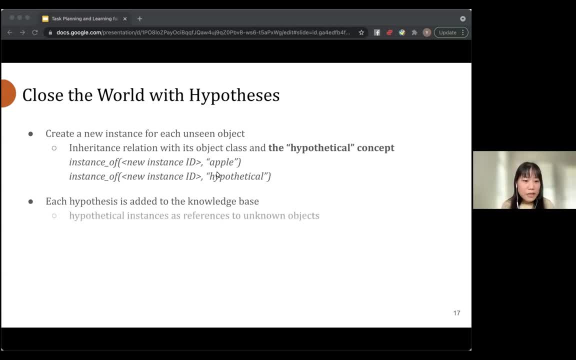 And then each hypothesis can be added to the knowledge base with hypothetical instances as references to unseen objects. So Like, if we think this apple can be in kitchen, then we can have this can-be-in hypothetical apple in kitchen. And it's important that when we describe the Golgoth condition, unseen objects are referenced. 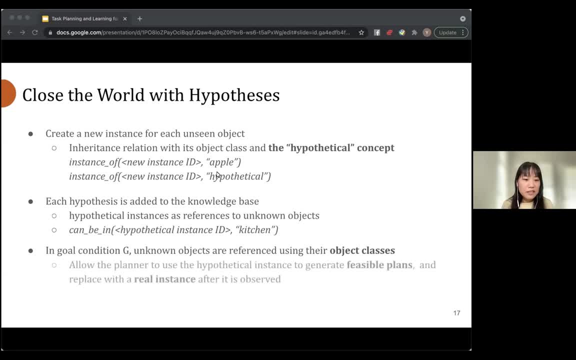 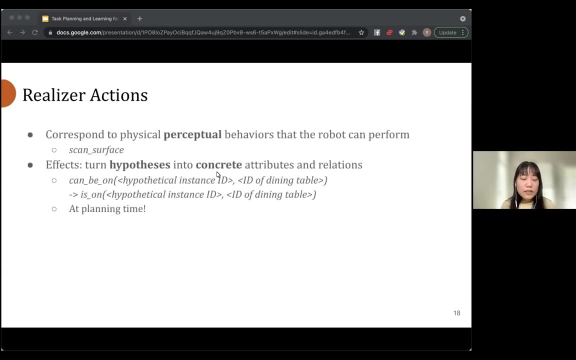 using their object class, not the instance. This allows the planner to use the hypothetical instance to generate feasible plans, but replace them with real instances afterwards And, like I said, the Realizer actions are modeled to correspond to physical, perceptual behaviors that the robot can perform like scan surface. 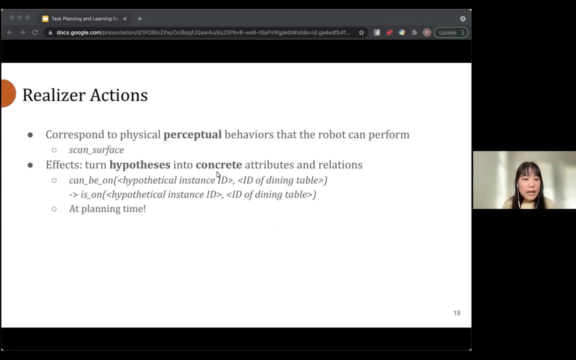 And we model the action effects to be that these actions turn hypotheses into concrete attributes and relations, Like if, before executing scan surface, you have can-be-on hypothetical apple on dining table and after in the planning domain, the effect of scan surface is that it turns. 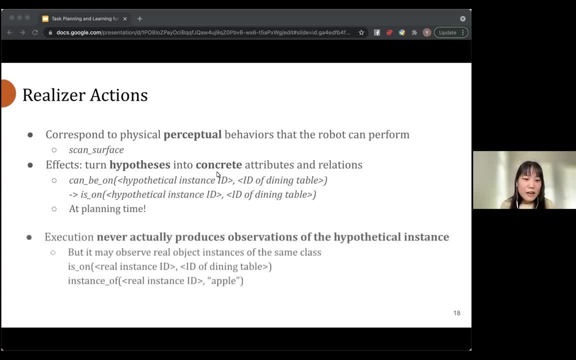 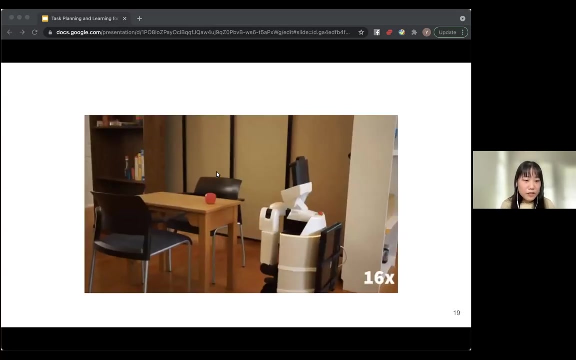 can-be-on to is-on, which is a concrete relation. However, execution will never actually produce observations of the hypothetical instance, but it will. People observe real object instances, maybe of the same class, maybe of some other objects, and they will all be populated into the knowledge base. 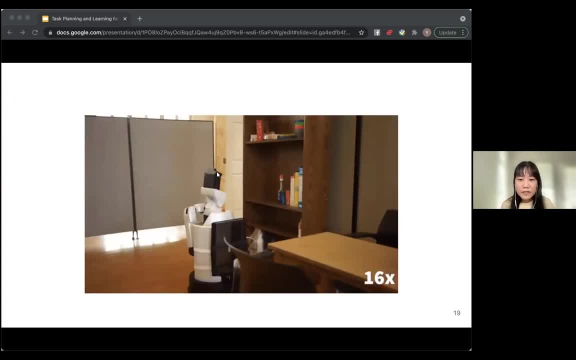 So here's a quick demonstration of a successful execution of the get-me-an-apple-from-the-kitchen task. The robot goes to every surface in the kitchen, replants if the apple is not there, until it finds the apple and picks it up. 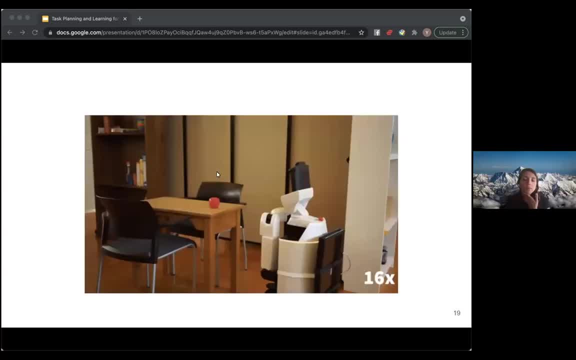 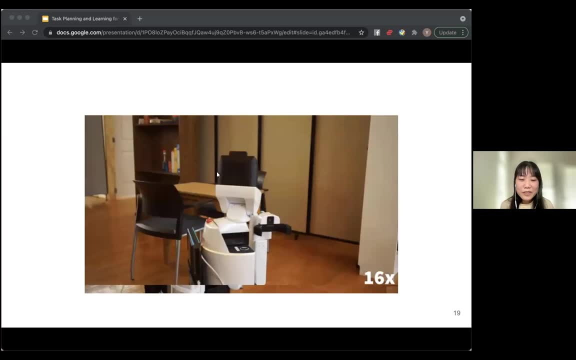 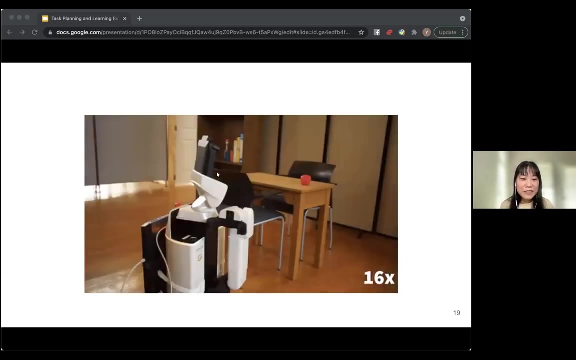 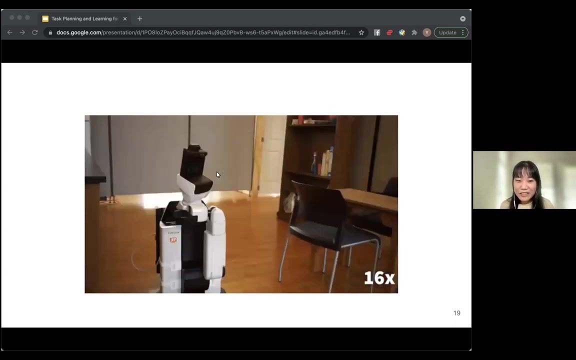 The default is in the nylo and opto through the ducts. Now here are two products that should be able tolerealize the product data to only monitor the necessary透ільки environment in its environment. Here we can see them, luckily. The goal was to create a model in which the ребbon can create Спасибо and I했는데 friends, or give you a Raz's Effects, Have fun, Thank you. You're welcome, Robin. 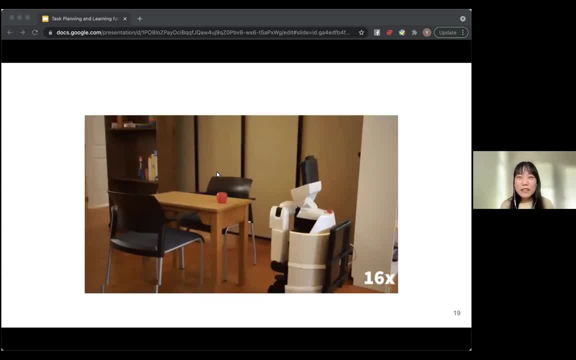 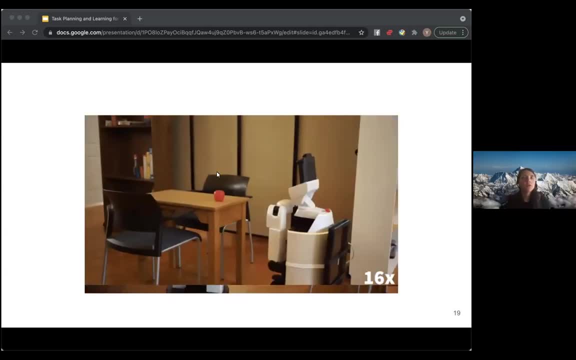 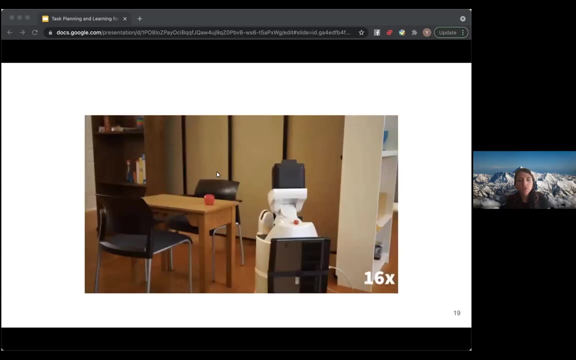 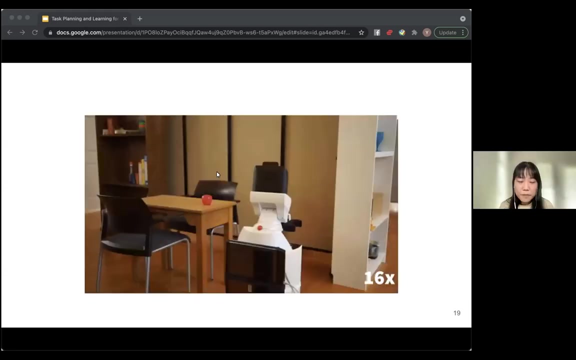 See you, Bye, Bye, Bye. Good question, Sorry of this is just focused on planning in this work, I see, And then do you use any machine learning models for incentivizing exploration or having agent better explore the scene, or this is planning-based? 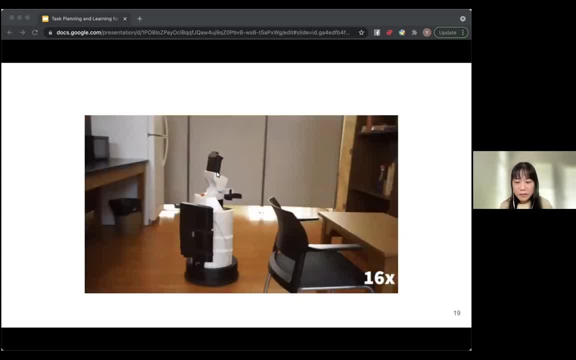 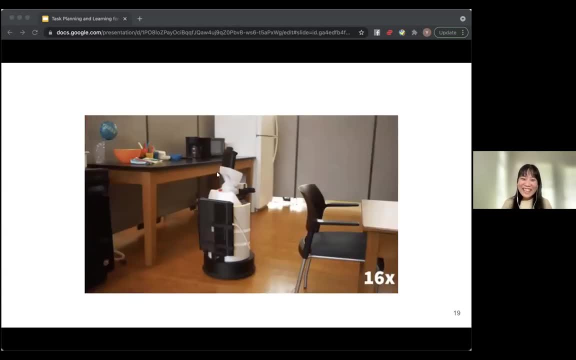 This part is planning-based. This is after the robot takes the user request, But I will talk about something that's machine learning driven to discover the environment. So very good question. So if there is no apple in the kitchen, we engage a diagnostic rule that attempts 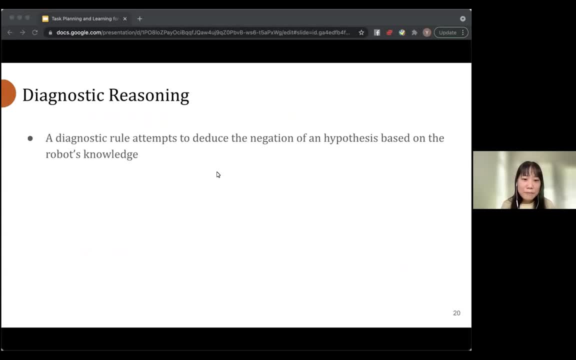 to deduce the negation of a hypothesis based on the robot's knowledge, For example, if a hypothetical object cannot be in the kitchen, if all surfaces have been scanned and no such object is found, And we formulate an optimization query which seeks to maximize the number of valid hypotheses. 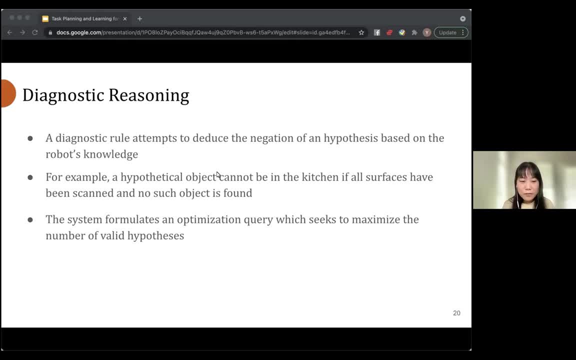 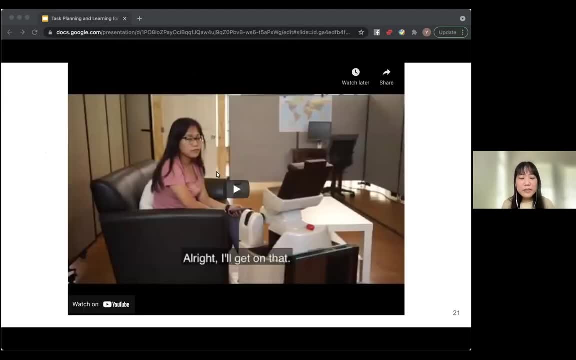 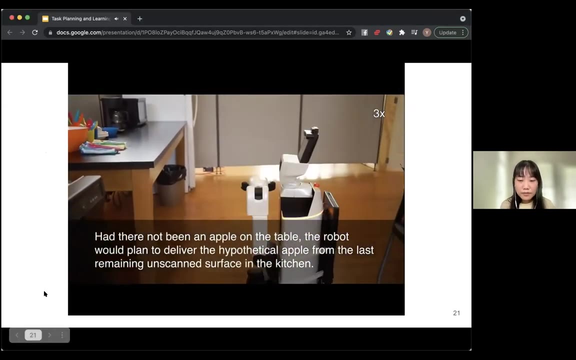 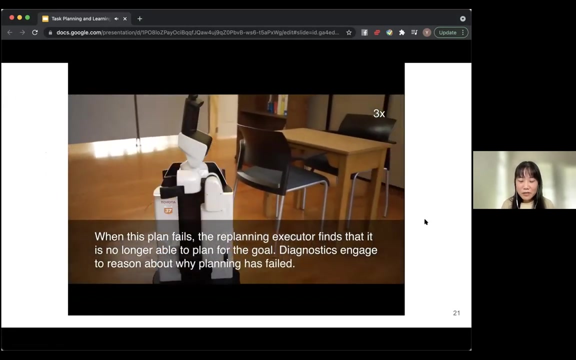 We were doing this with answer set programming and the Klingle solver So this was kind of straightforward to do with the optimization query, And here I will show a demonstration of using this diagnostic reasoning rule. I think maybe I forgot to enable sound. I want to share the screen so it will be captioned. 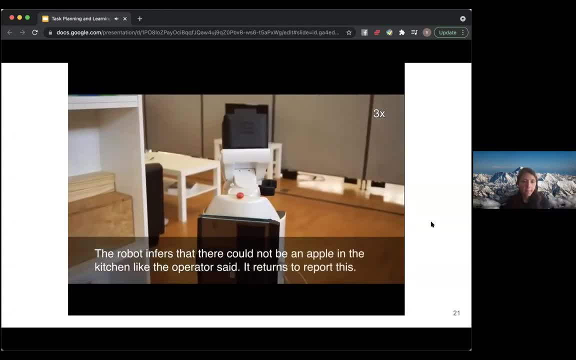 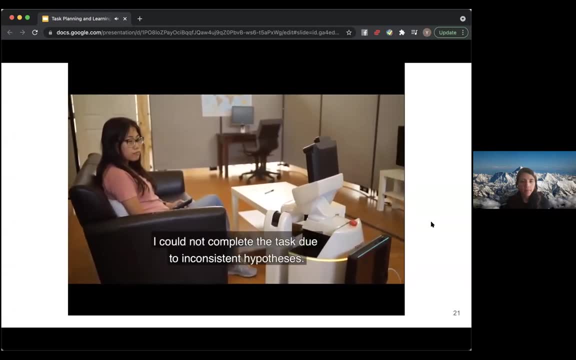 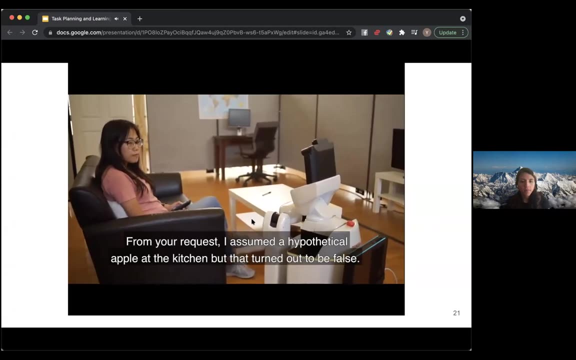 No, you did. We can hear it. Yeah, Cool. I could not complete the task due to inconsistent hypotheses From your request. I assumed a hypothetical apple at the kitchen, but that turned out to be false. So, OK, Very simple demonstration there. in summary, 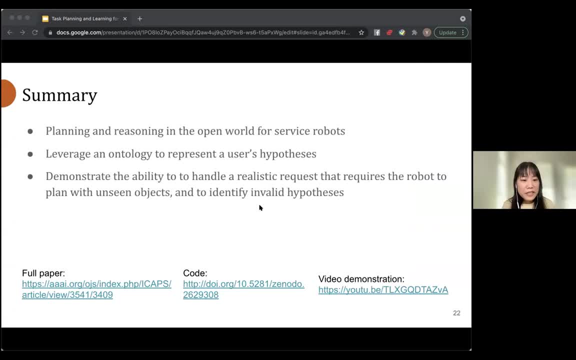 OK, So OK, Very simple demonstration there. We propose the approach to do planning and reasoning in the open world for service robots that represent the user's hypotheses to enable feasible plans to be generated and re-planning or monitoring during a plan execution, And we demonstrate the ability to handle a realistic request. 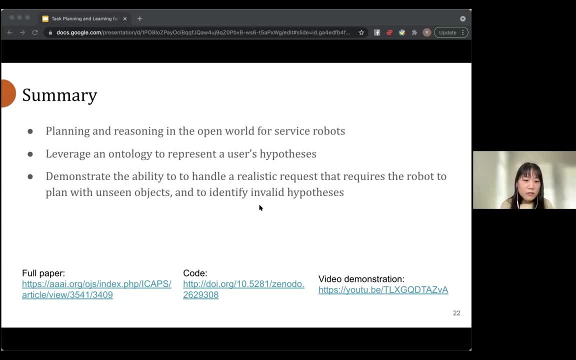 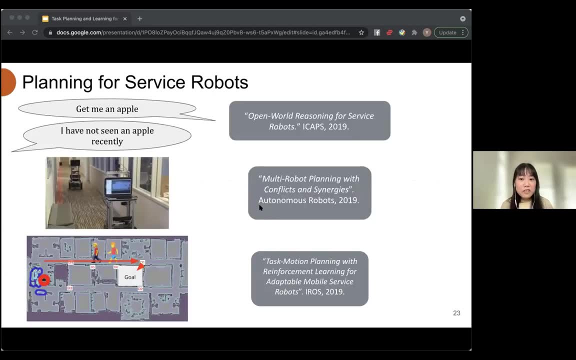 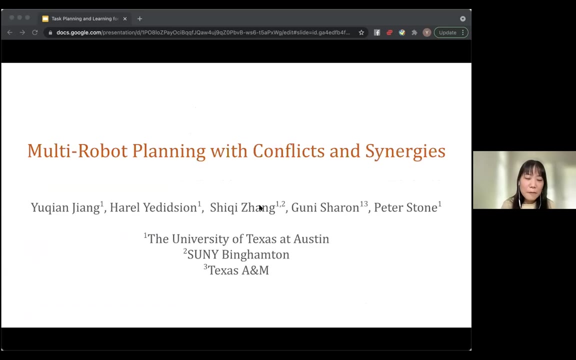 that requires the robot to plan with unseen objects and to identify invalid hypotheses. So Now we move into a larger building environment where there are multiple robots moving around and completing user requests. This was drawing work with Harao Edishin Chiqi Zhang. 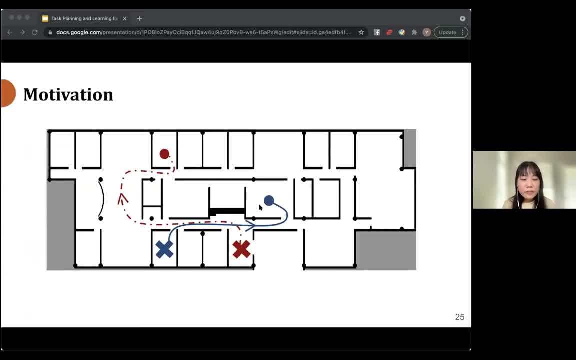 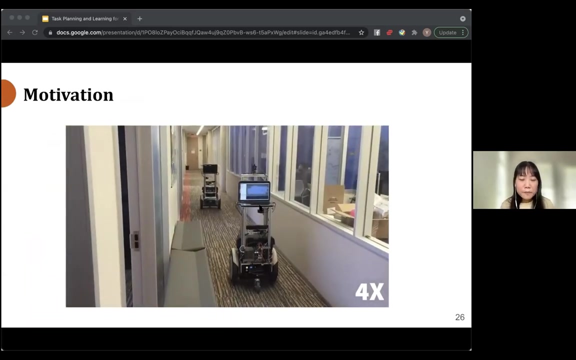 Guni Sheran and Peter Stu. This is just a visualization of two robots- actually discrete plans, but visualized this way- And, as you can see, they were likely to meet each other in the corridor, And sometimes the corridors are not wide enough for them. 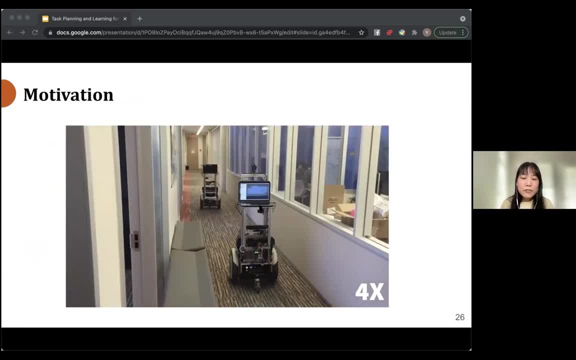 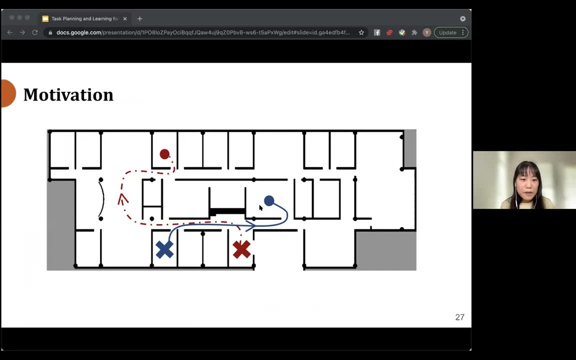 to pass each other And without coordination, they will just see each other as large obstacles and both will turn around. However, if we try to address this problem at the planning time, we can predict that there will be a collision, And we can. 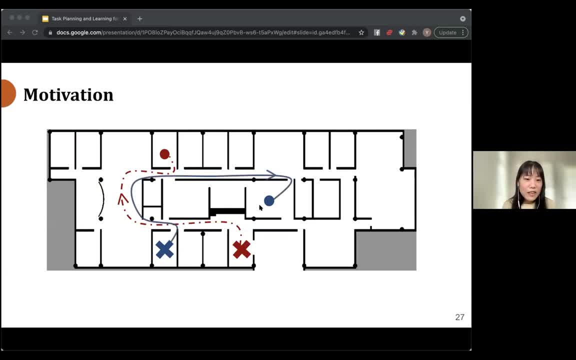 OK, We can adjust the robots plan so that it adapts to the other robot's plan. They do not have this conflict anymore, Or they could realize scenarios like if they both need to go somewhere and their shortest path may involve opening different doors. 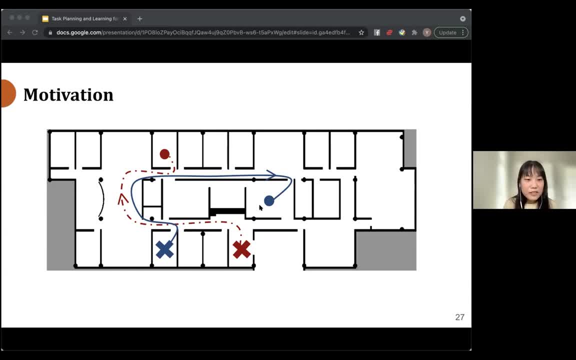 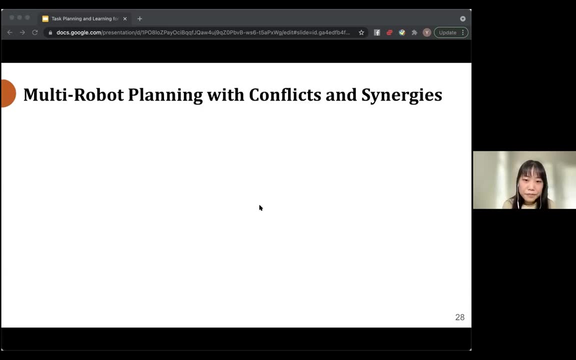 But if they know about the other robot's plan, one of them could go ask for help And one of them could just wait for the door to be open, and therefore minimizing the total plan cost of these robots. And so we formalized the multi-robot planning. 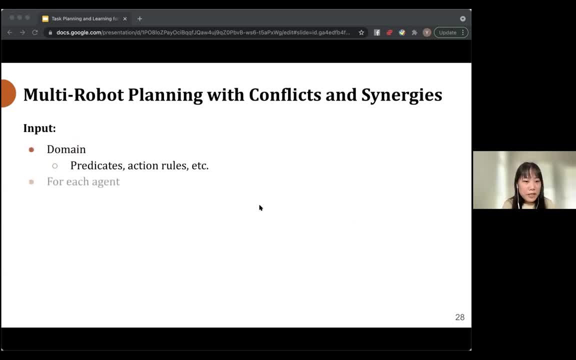 with conflicts and synergies problem. The input is again the planning domain And for each agent we have to model the distribution of action duration, since robots can easily get delayed by other obstacles, And we want to be able to do that. 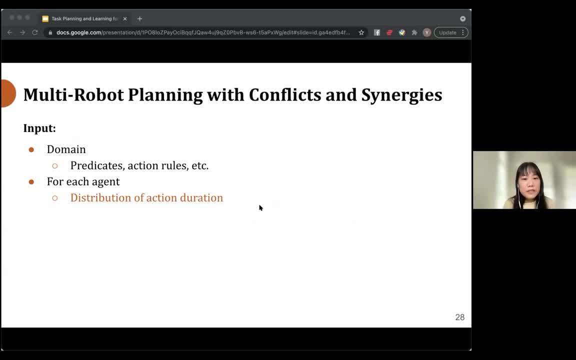 We want to be able to predict basically the probabilities of how some synergies or conflicts can happen And we need a cost model of conflicts and synergies And, of course, initial state and no state, And the output is the set of plans, one per robot. 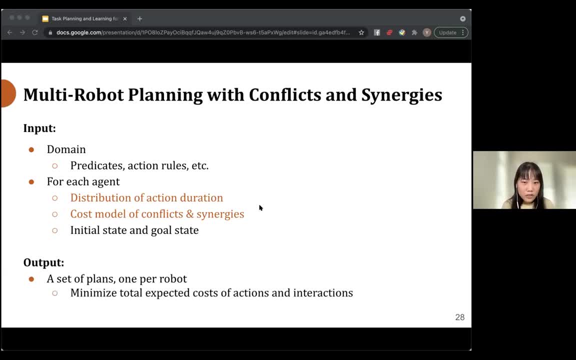 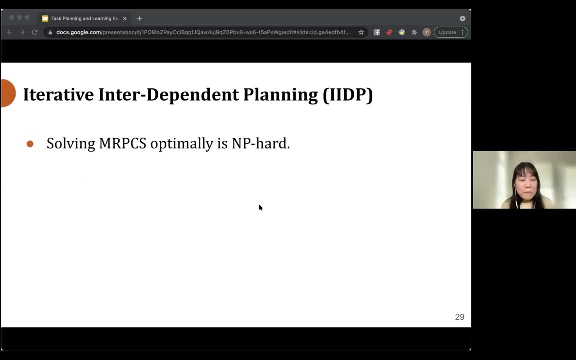 to minimize total expected costs of actions and interactions, including conflicts and synergies. And solving this problem optimally is NP-hard And therefore we want to avoid going into the combined state space of all the robots. That way we can scale to the number of robots. 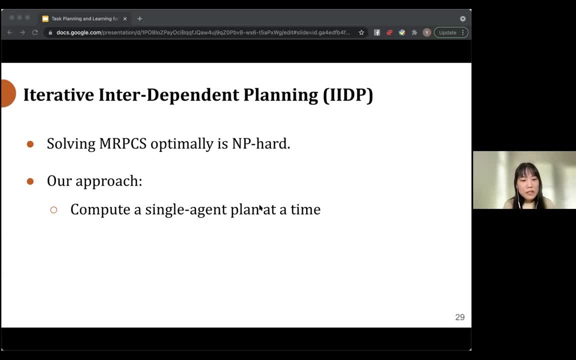 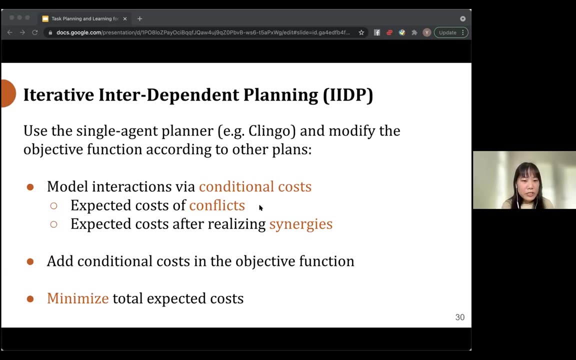 So our approach at a high level is to compute a single agent plan at a time that's dependent on other robots' plans, And so we never have to consider the combined state space, And we do this by modifying the objective function according to other robots' plans. 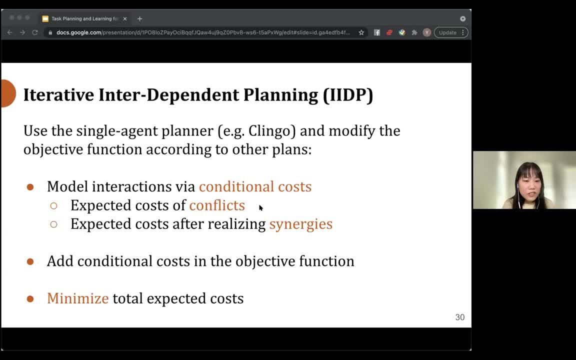 Basically we model interactions via conditional costs, including expected costs of conflicts and expected costs after realizing synergies, And then we can add these conditional costs into the objective function And we minimize total expected costs for each robot. As a simple example again with the two robots: 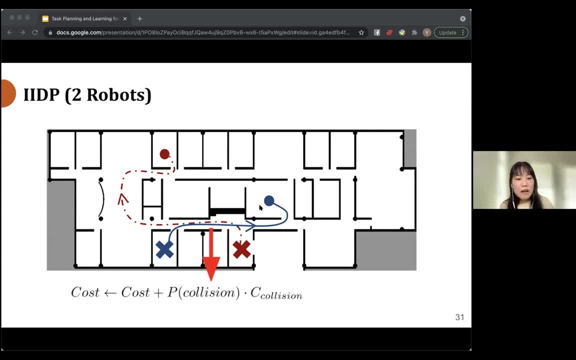 we will see that they might have a conflict And we can model the probability of this collision times like a predefined cost of this collision to each of the robots' planning problem, And then the blue robot might discover this other path that does not have this conflict, with lower total expected costs. 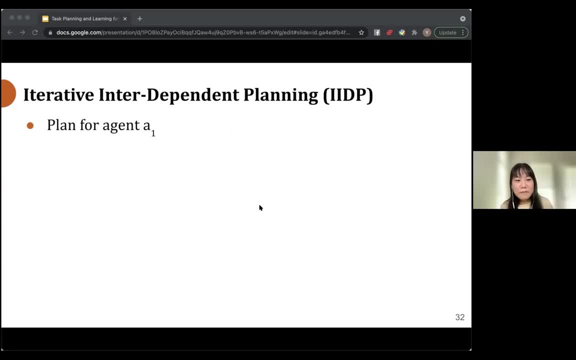 So there's this very simple algorithm for iterative interdependent planning. We just plan for agent 1. And plan for agent 2,, dependent on the plan of agent 1, and so on, And the problem with that is the ordering of the agents matters. 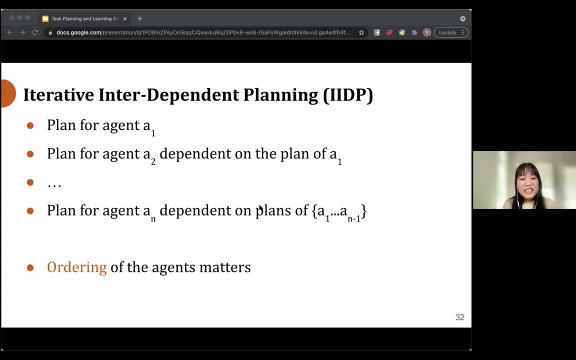 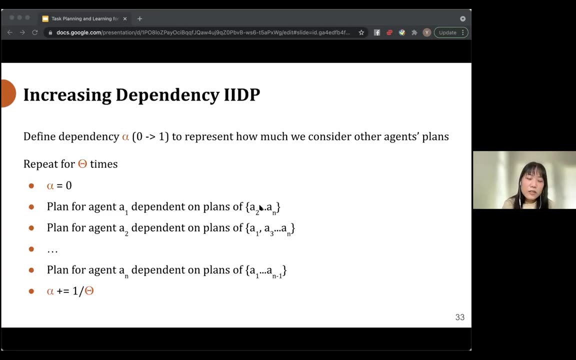 Like, for example: as you can see, agent 1 will never have a chance to adapt to the other robots' plans, And if that's the one agent that's causing all the problems, causing all the conflicts, we'll never have a chance to correct that. 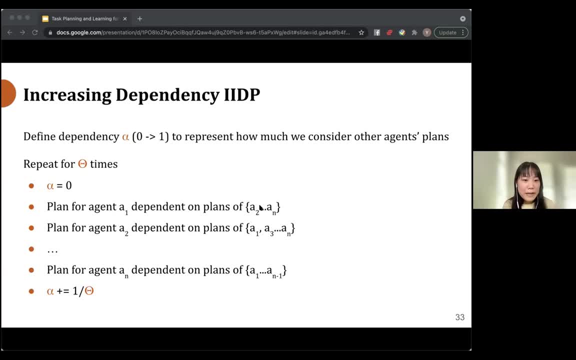 So we proposed an algorithm. We have a algorithm called increasing dependency, IDP, where it's inspired by other approaches, But basically we have defined the dependency parameter alpha to represent how much we consider other agents' plans, And in each iteration we increase this alpha. 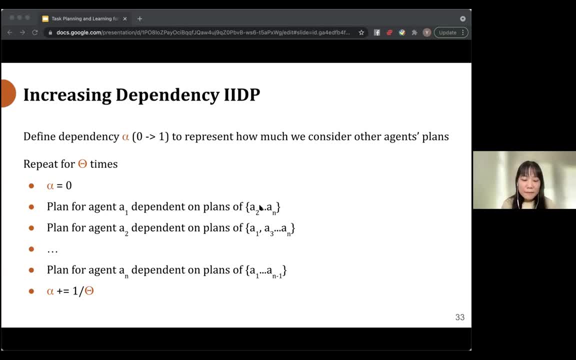 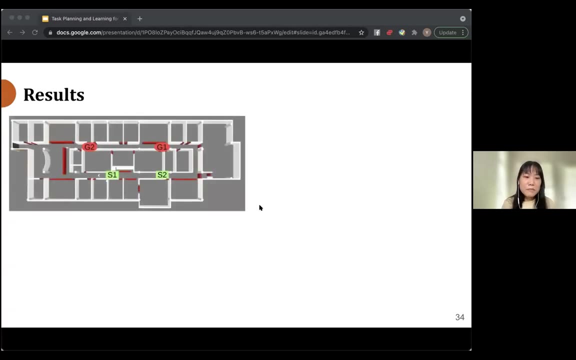 so that we increasingly consider other agents' plans And the effect that it achieves is the agent that has the lowest cost to switch to a different plan will switch first And then the ordering sort of gets resolved. naturally We have some results in the Gazebo simulation with two robots. 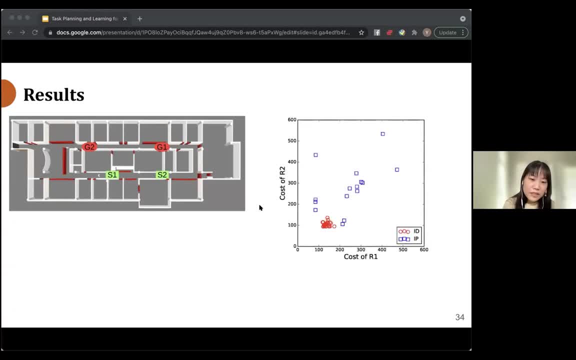 And it's sort of straightforward to look at. Here we plot the cost of robot 1, the cost of robot 2.. The red circles represent the increasing dependency algorithm's results and the blue squares are from just planning independently, And we can see that having this increasing dependency 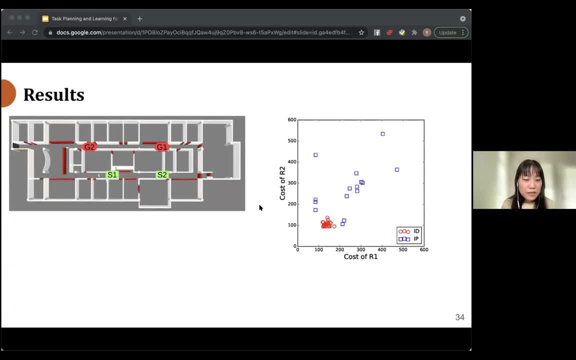 coordination makes them sort of avoid those conflicts and have lower total cost and lower variance. This approach has also been implemented on the real beta by bots, And here is an example where the two robots realize the synergy. One of them goes to ask for the door to be opened. 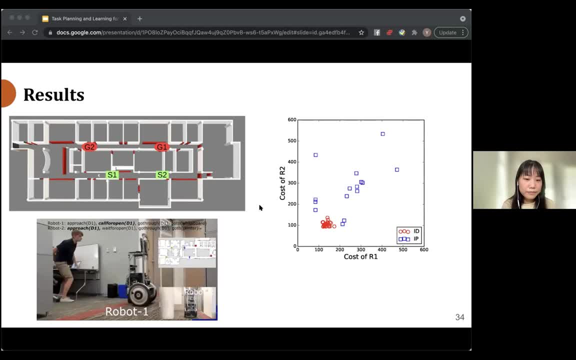 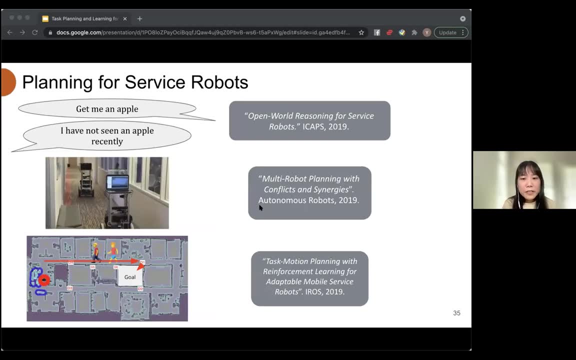 And the other one just follows through. So that was the work on multi-robot planning with conflicts and synergies. Next, we consider the problem of task motion planning in a dynamic environment. This was drawing work with Fengtai Yang, Xu Zijian and Peter Stu. 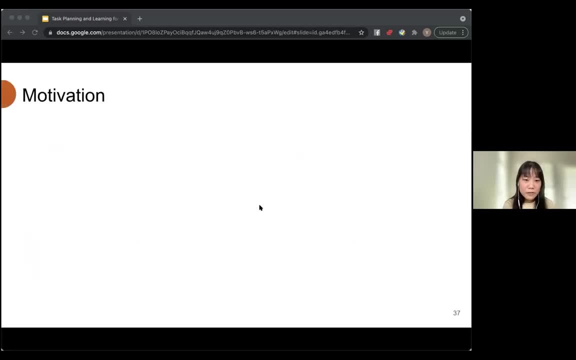 So again, we're considering mobile service robots in large environments like buildings And to plan for tasks like deliver coffee to Alice's office or to work on a project with them. And then we consider the problem of task motion. we not only have to plan at the symbolic level, but also need to integrate a motion planner that generates paths in a continuous space. 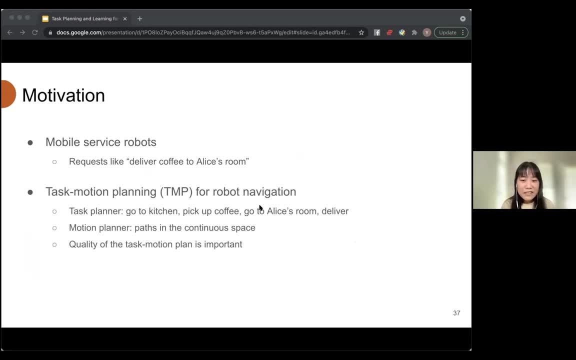 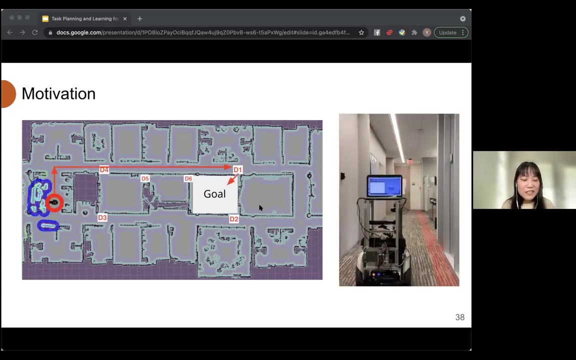 Usually, such feasible plans are not unique and we want to minimize the plan cost so that the coffee is still hot when it gets there. Why is this a challenging problem? Well, first of all, there could be many feasible plans. In this case, there are many doors to go into the target room, and the environment changes. 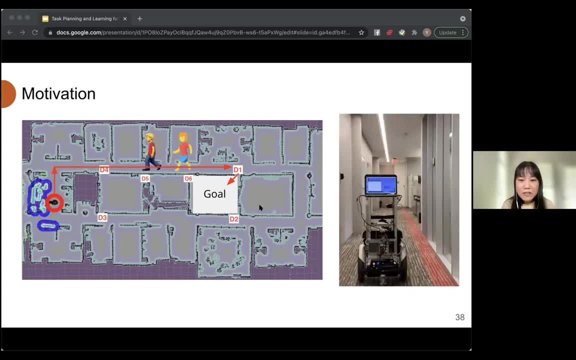 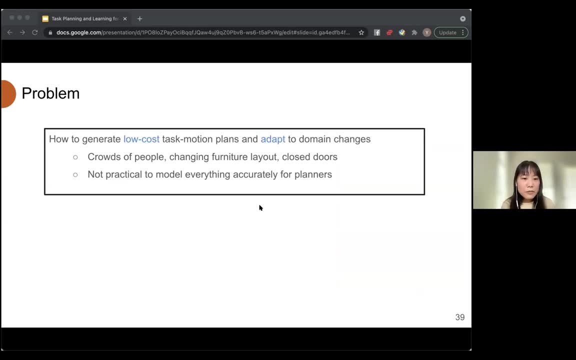 Some doors are always closed and there could be crowds of people moving, So the problem which we're trying to solve is how to generate low-cost task motion plans and adapt to domain changes, such as crowds of people, changing furniture layouts and closed doors. 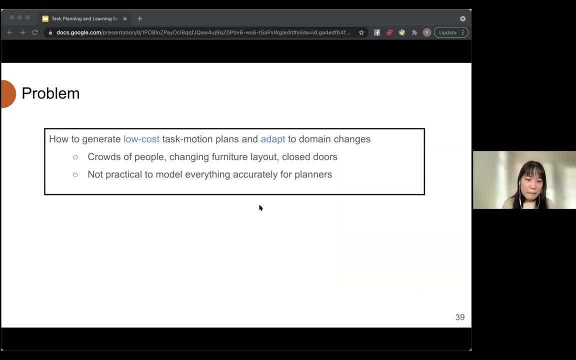 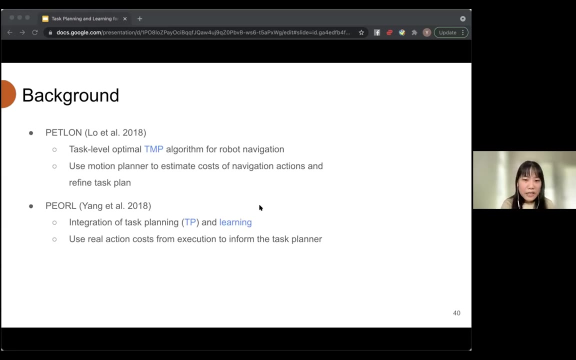 which are not practical to model accurately for people. So we have two problems here at planning time And basically there were two compelling approaches. One is the Task Motion Planning Algorithm for robot navigation. Basically it uses the motion planner to estimate costs of navigation actions. 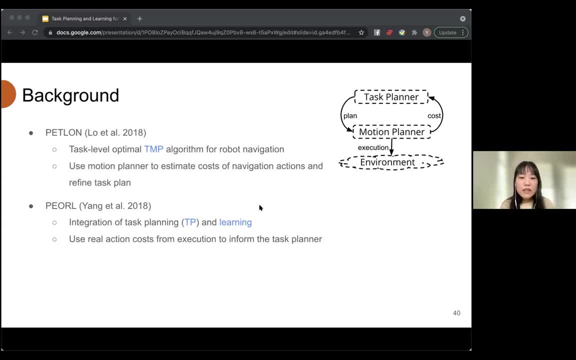 and the task planner uses that information to iteratively improve the task-level plan. There has also been integrations of task planning and learning learning. This example approach here uses real action costs from execution to inform the task planner. So what we wanted to do was basically to combine both of these ideas. 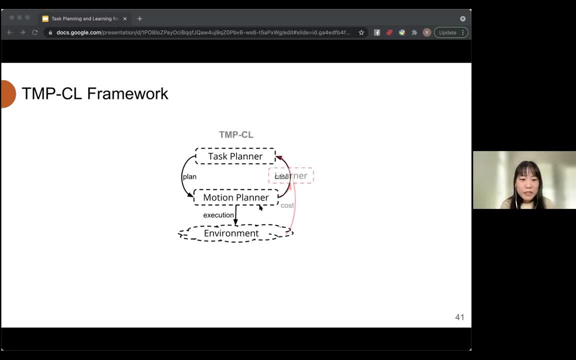 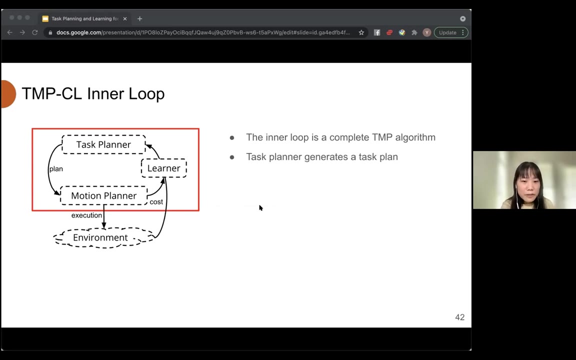 into one framework. In this framework that we proposed, there are two planning and cost learning loops that receive action cost estimates from both the motion planner and the environment. Here we look at the inner loop. It's a complete task. motion planning algorithm. First, the 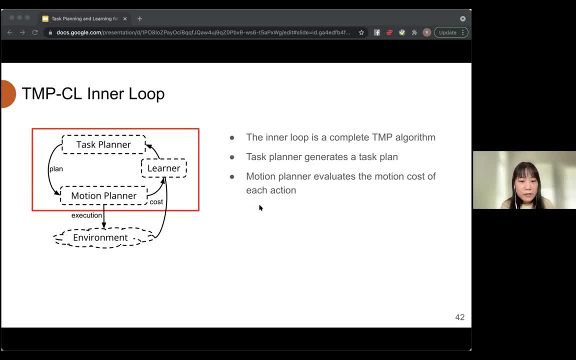 task planner generates the task plan, then the motion planner evaluates the motion cost of each action and then the learner updates the costs for the task planner And this loop terminates when the task planner cannot find a plan with higher quality or lower cost with respect to the costs estimated by the motion planner. 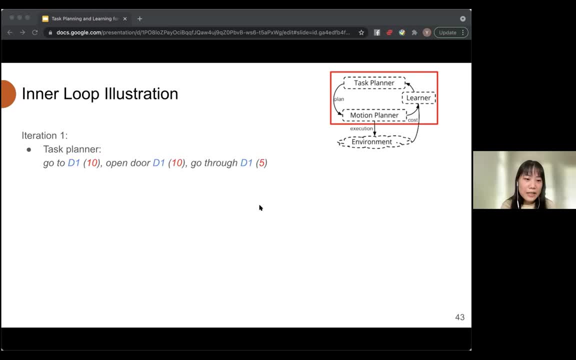 And just to illustrate there's a simple example. The task planner might say: go to door one, open door one, go through door one, And the numbers in the parentheses are initial costs as mates of those actions And the motion planner will evaluate each of those navigation actions. 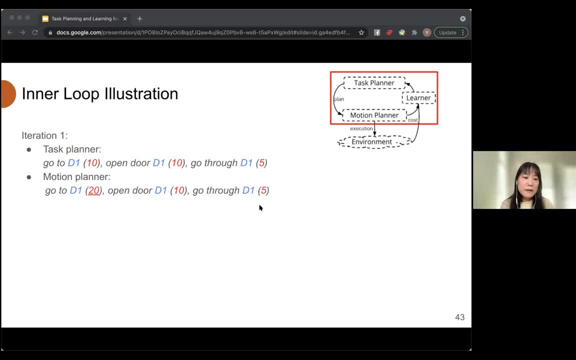 and might discover that going to door one, the path is longer than expected and it will take in like two minutes. And then the next iteration: the task planner can reevaluate all the feasible plans and finds another one like go to door two, open door two or go to, And then 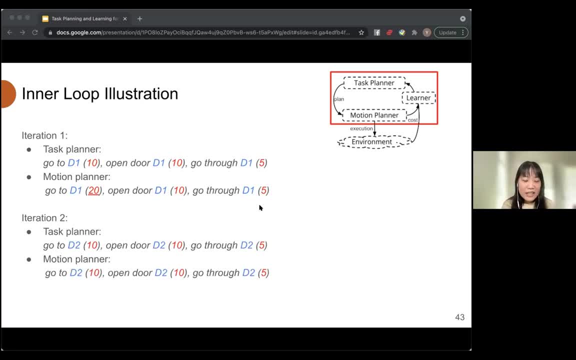 ballerina planner can evaluate all of them again and maybe this time will confirm those estimates and the task planner won't be able to find a better one and the inner loop terminates Did the conditions that were draftedordum 0 are true. Yes, it's true, And has there been a future basis for other information that very mature? So what we're also measuring, we're doing later on, is to evaluate based on their own experiences. One could actually get up-to-date results on the general basic by using the 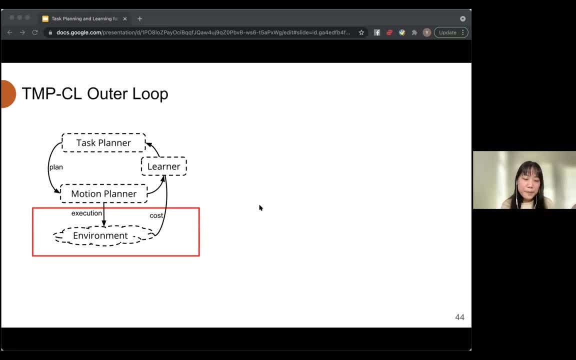 program. the question matter character in thereetruth, But then Are some communication and step-by-step experts would 자주 need to answer these. question the plan: um it will get executed in the environment and the learner updates action costs um using experiences from those executions and then the inner loop can use the learn costs. 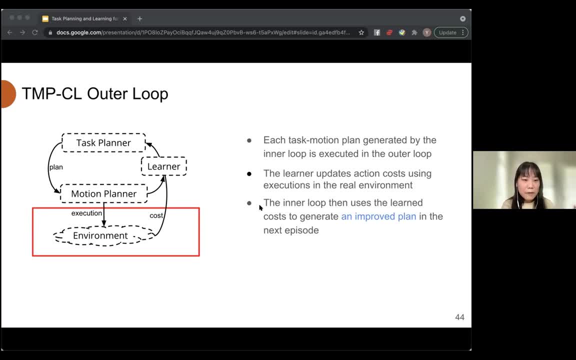 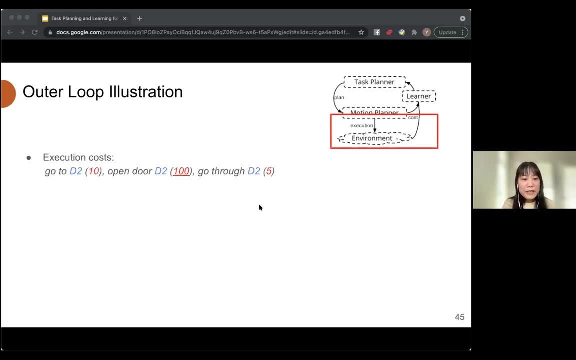 to generate an improved plan next time. it's required to plan. so to continue, our last example maybe: opening door two takes a very long time and the learner will update the cost of those actions and then the inner loop has motion planning can decide on a different plan next time. 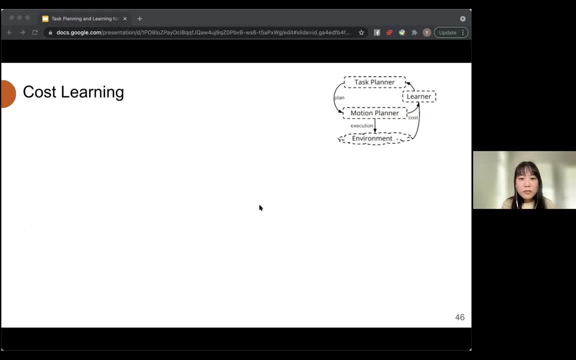 so um. the essential component here in this framework is the learner, which integrates feedback from both motion planning attempts and real execution attempts. basically, we treat each action cost it receives as a sample cost and use it to estimate the true cost of that action by an exponentially weighted moving average. next we evaluate the tmpco approach. 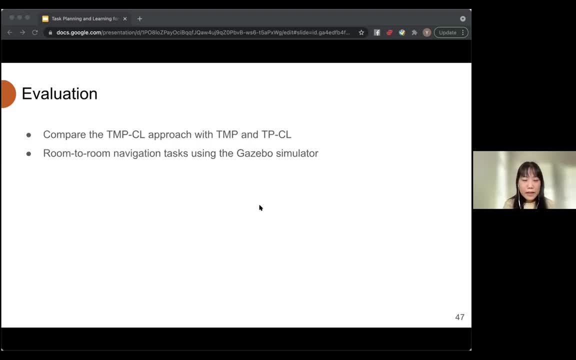 with the just the task motion planning, or task planning with cost learning approaches that i mentioned earlier. um, the experiments were conducted in a room to room and place room-to-room management program to create the model for the action cost of that action cost. just a customer planning or task planning with class learning approaches that i mentioned earlier. 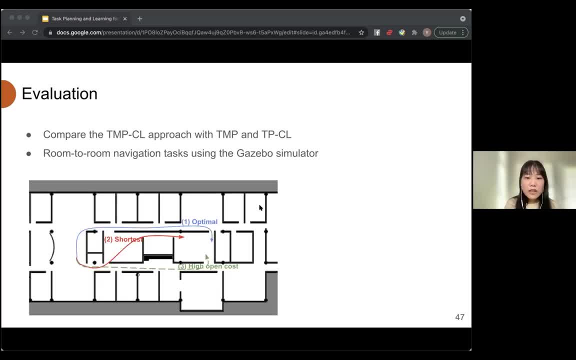 the experiments were conducted in a room to room and place, room to room and place, the method of the action room navigation task using the Gazebo simulator And basically the set up is that there are three competitive plans of this task And the environment is different from what's modeled, but it has motion planner. 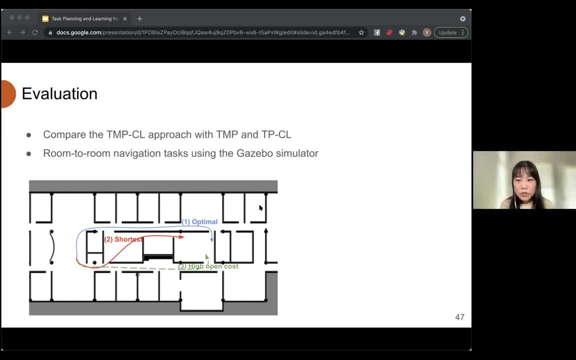 So the robot needs to adapt to the optimal plan, which goes through the door that's usually open, And the second plan has the shortest navigation distance, but it goes through a bunch of doors that are usually closed and require additional time to open. And then a third plan is also short in navigation distance, but the door takes a long time to. 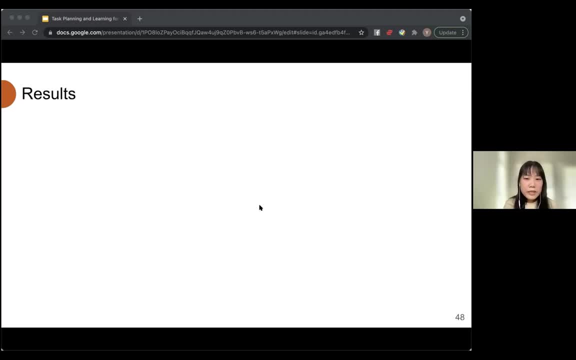 open. We ran all three methods for 40 episodes, repeated 50 times. Here are the learning curves. As you can see, TMPCL- the blue curve, and TPCL- the green curve. both converge to the practically optimal plan. 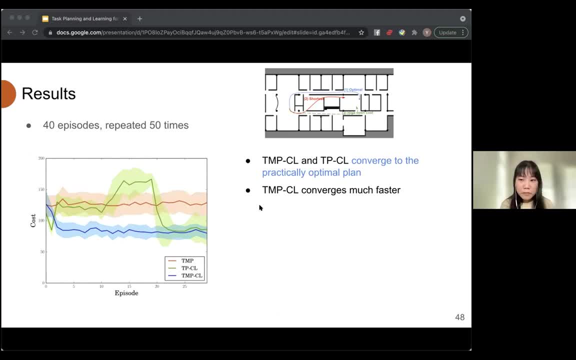 But TMPCL. we're able to come Converge much faster with the help of the motion planner. TPCL without the motion planner has higher variance and a simple TMP planner does not learn from executing in the environment. To visualize the results better, we plot the distribution of how many times each of those. 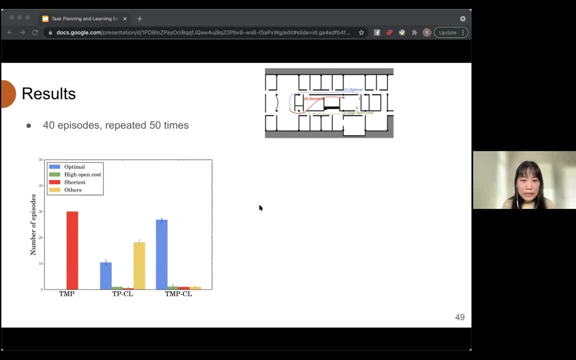 competitive plans or other plans are executed by each method And again we see that TPCL has to try out many logics. So the real robots only execute the planned plans, but TMPCL does not learn from executing in the environment. So we can see that TMPCL has to try out the planned plans and TPCL executes the planned. 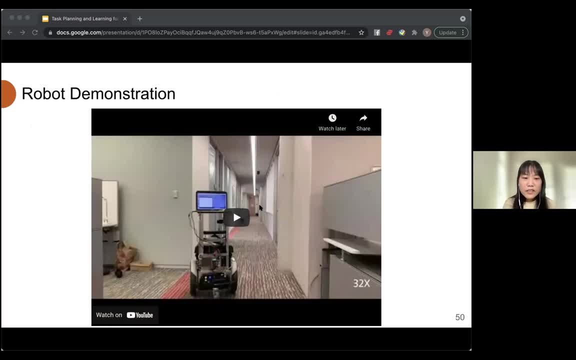 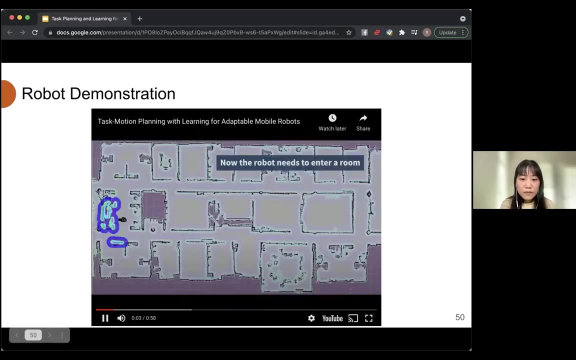 plans with the shortest navigation distance, And here I will show a VIL demonstration on the real robot. The setup is similar to what happened in the Gazebo experiments: Doors take a long time to open and some places are crowded. And the robot has access to this map. 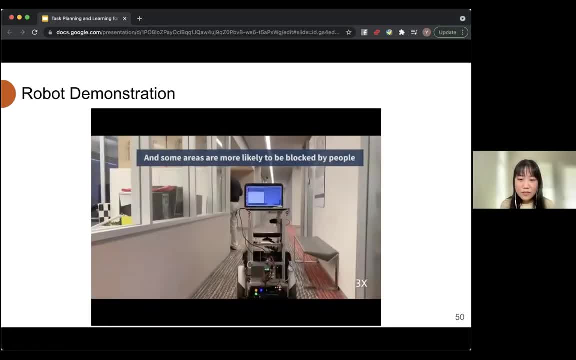 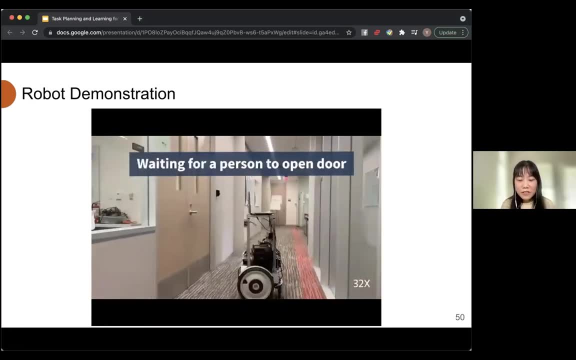 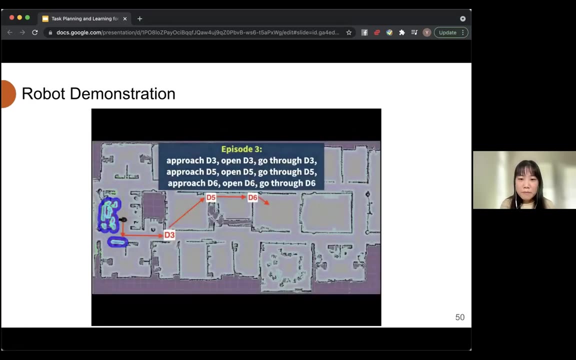 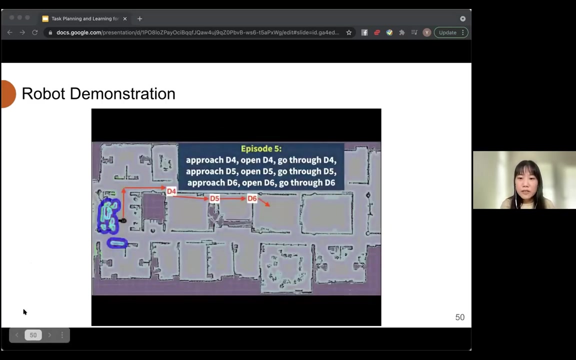 Yes, hand right. Yes, The only thing that it doesn't know is, like those factors that could influence how long it takes to execute each plan. So the rest of the video is basically a quick run through of those action executions happening the outer loop of the framework. 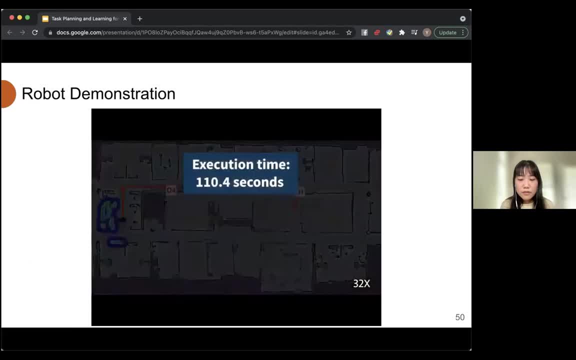 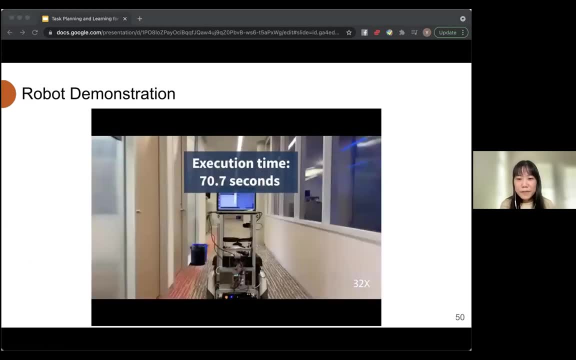 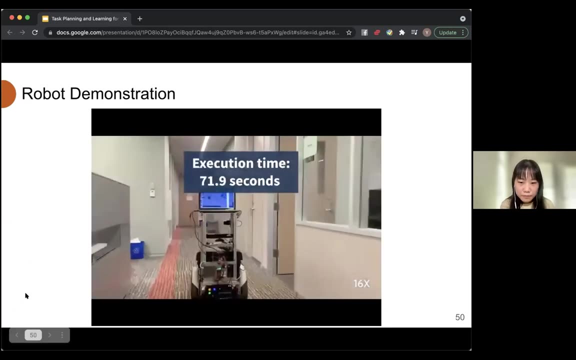 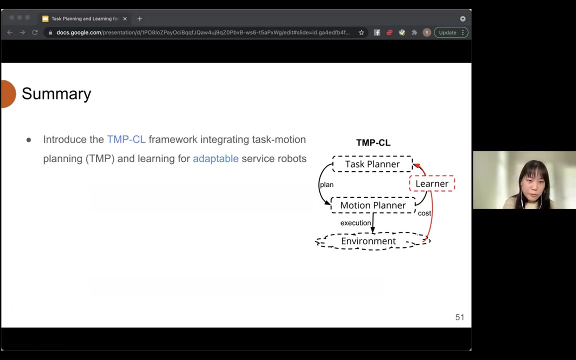 And basically, by the seventh time it's executed, it was able to adapt to the best plan. Okay, In summary, we introduced the TMP-CL framework, integrating both past motion planning and learning for adaptable service robot navigation, And experiments show that the framework combines the strengths of both past motion planning and 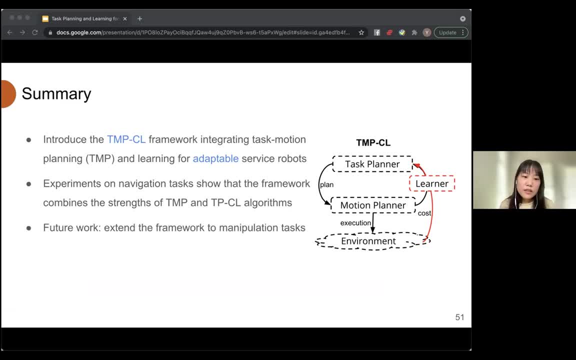 task planning with cost learning algorithms And in future work we would like to extend the framework to mobile manipulation tasks, which has a different set of challenges. But the high level idea is that we want to learn from both motion planning attempts and real execution experience. 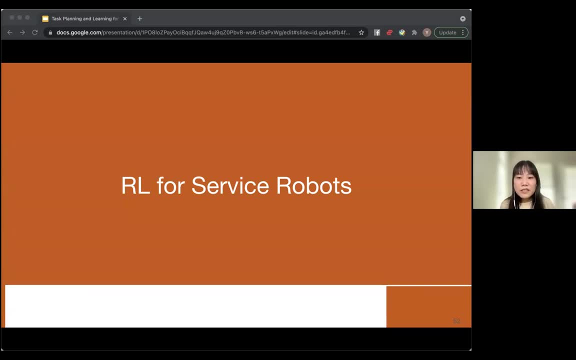 So that was the first part. I would just quickly introduce this other direction of our research. in general, we aim to develop RL methods for suitable service robot problems, especially continuing tasks that are understudied but not uncommon, in long term deployments of service. 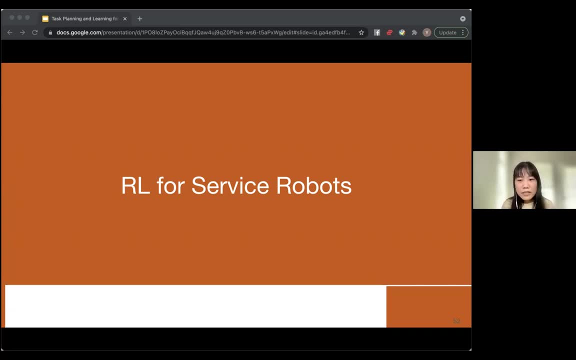 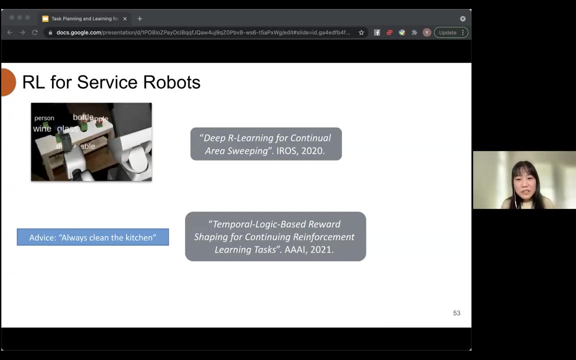 robots, And we also want to leverage reasoning and planning to improve sample efficiency. In the interest of time, I will not go into details about these papers And for this first one, at the high level we're interested in this continuous error-sweeping problem, where the high level goal is, as mentioned earlier. 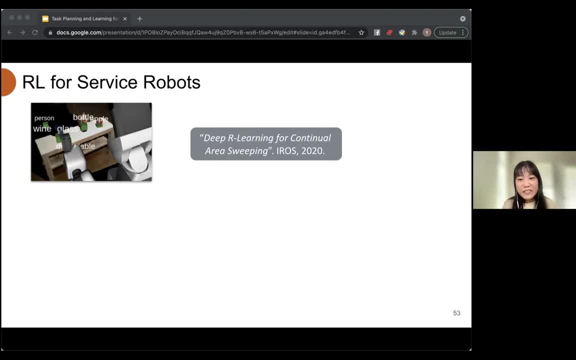 that the robot goes around the environment, service the environment efficiently when it does not have an active user request. So it has idle time so that it can perform cleaning or updating its knowledge base. And we formalized the continuous error-sweeping problem as maximizing the average reward in a 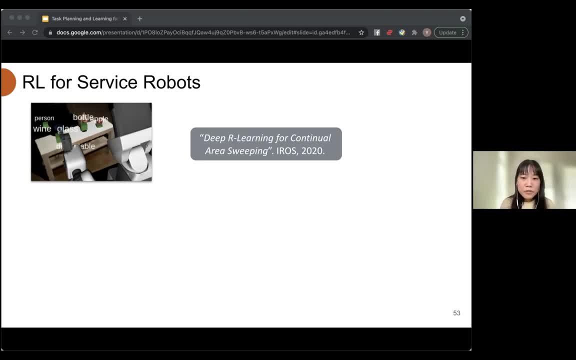 semi-Markov division process And we introduced a deep RL algorithm for such a setting And that's just a cute animation for the setup of this problem, basically. And the continuous error-sweeping problem motivated us to study continuing tasks and the average reward setting better. So that leads us to the next contribution. Again, I'm not going, 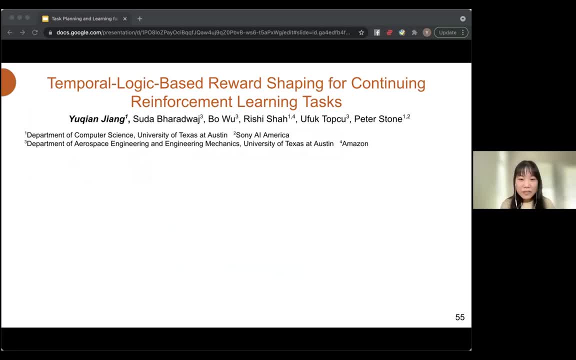 to details, But I guess just to introduce the problem. in continuing tasks it's particularly important to avoid long stretches of informative exploration, And reward shaping injects advice and guides exploration by providing extra rewards. Since manually writing down those rewards can be non-trivial, we wanted to automate construction of the shaping function from like a user given a 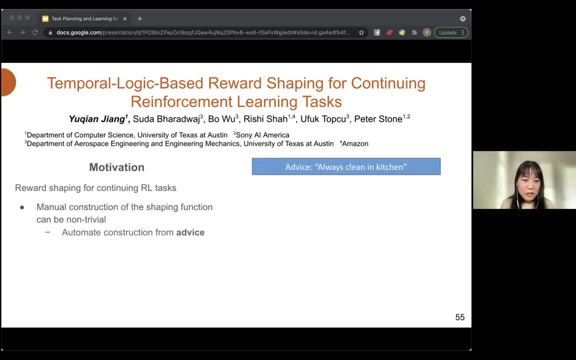 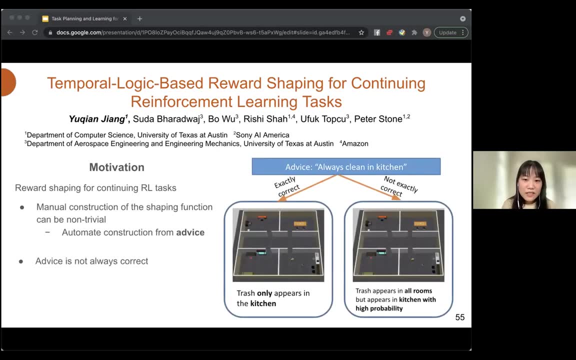 device, But advice is not always correct. We also want to ensure that imperfect advice cannot prevent learning the real task, And one approach that gives this guarantee is potential-based reward shaping, which guarantees that the optimal policy is not affected, but it has not been studied in the average reward setting. So in this work we first extended 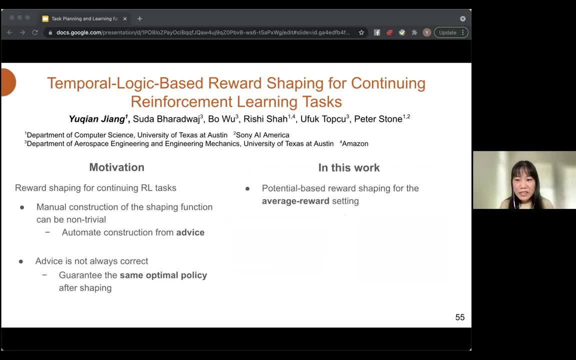 the potential-based reward shaping to the average reward setting and provided an approach to construct the potential functions from temporal logic specifications, And our main technical results were of proof that the optimal policy can still be recovered with this potential-based reward shaping in the average reward setting and empirical evaluations showing that the method 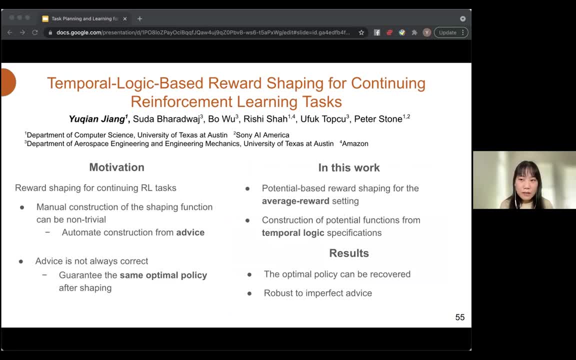 improves learning performance and is robust to imperfect device. How do you process the advice Basically? is it a template-based sentence or can it be in any form? It's template-based. We sort of assume that it's already in a form of temporal logic specification. like: always clean a kitchen. So those are things. 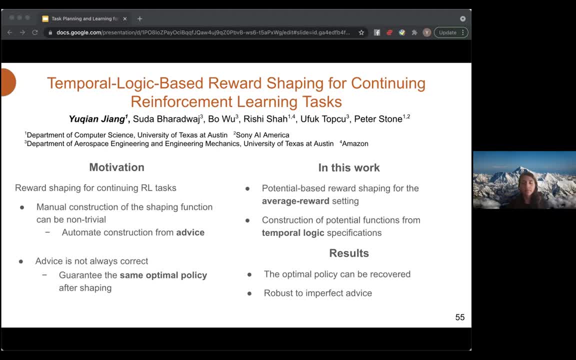 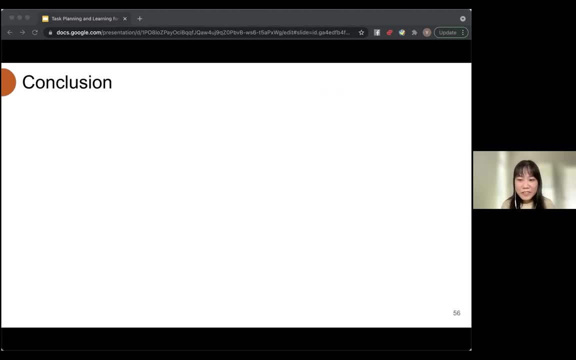 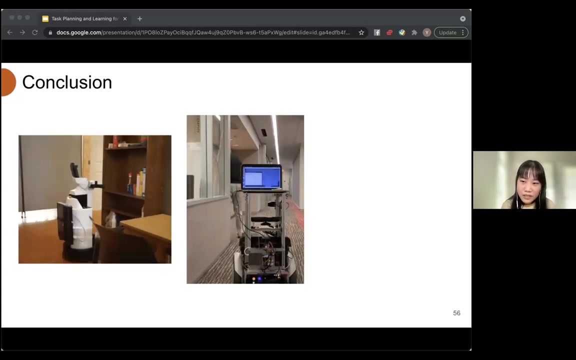 easy to yeah model. That was our series of ongoing efforts towards building high-level planning functions of general-purpose service robots. These methods will enable robust and adaptable task-motion planning in dynamic environments, as well as continue air sweeping as a background task to efficiently obtain the robot's knowledge In cases where multiple robots operate in the 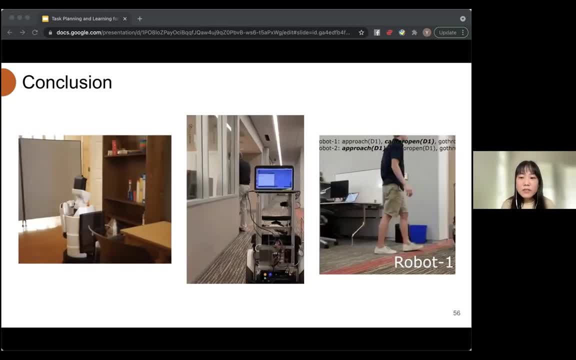 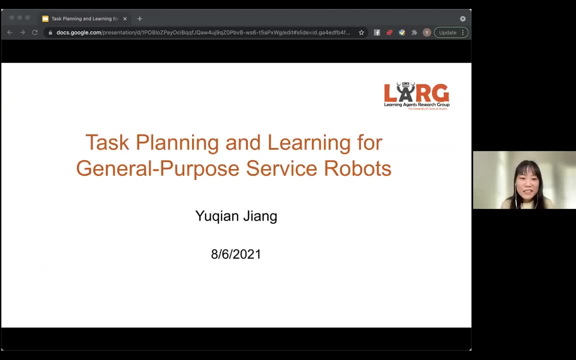 same environment, they're able to adapt the high-level plans to avoid collisions and to form synergies. and um, that's um. that's all i. i guess i have lots of time for questions, so, yeah, thank you very much. uh, thank you, this was very interesting and you did a great job, uh, explaining it in a very 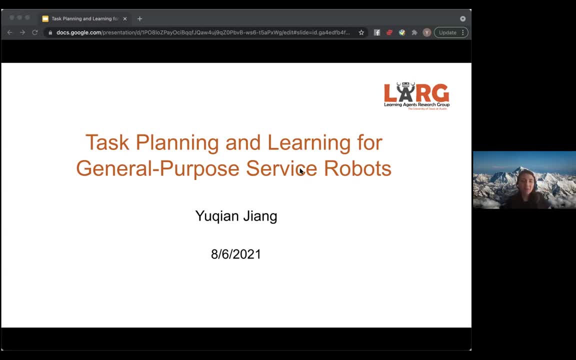 understandable way for people who are more on the computer vision and embodied ai side and not very familiar with the uh, the motion planning. yeah, thank you so much. do we have any questions from the audience? cool, i, i think i um, i ask a question, man, uh, so i was wondering um for uh, for the? 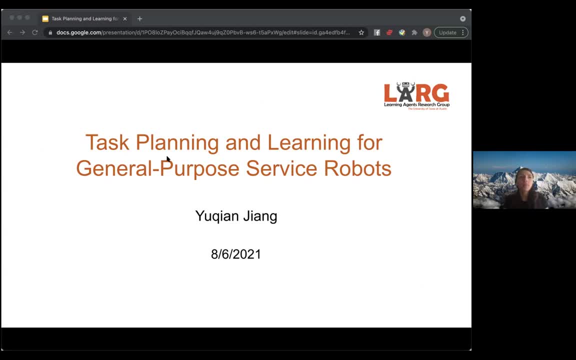 exploration phase for the beginning, where um you still, uh, don't um, um, for, for i think it was the first project that you mentioned- that um, if you are looking for an object that the agent has never seen? um, so the exploration using rl methods have been studied a lot in the embodied ai. i was wondering. 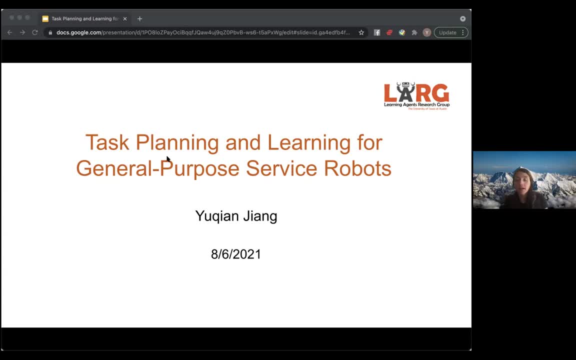 if you've tried any of those to see how well it works in this setup, or whether, um there is any benchmarking against any of the rl methods or learning approaches. i see, so i guess those methods will work well. um, if you don't already have hypotheses from the user, um or or like if